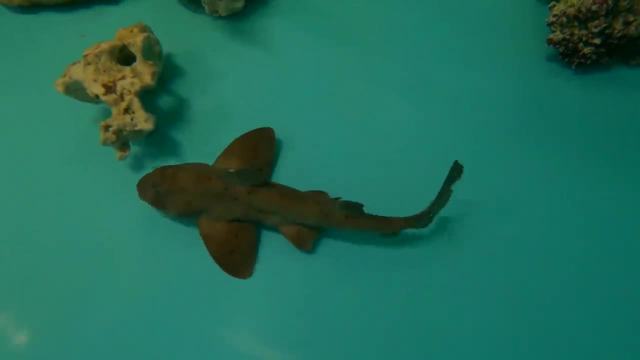 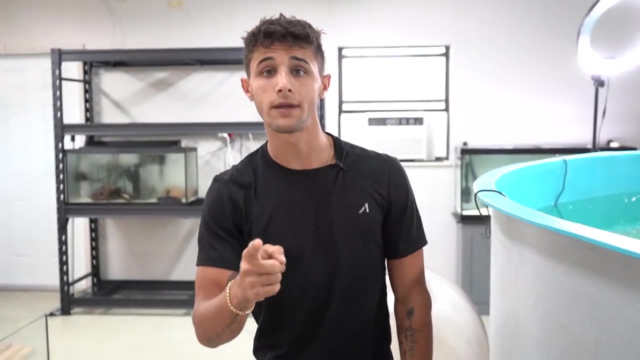 stingrays, sharks, you name it. It's pretty much in here, But everything in the saltwater pond is doing awesome. I've been uploading a lot of Instagram stories, feeding them. If you don't follow me on Instagram, popping up right here on the screen, make sure you go follow me so you don't. 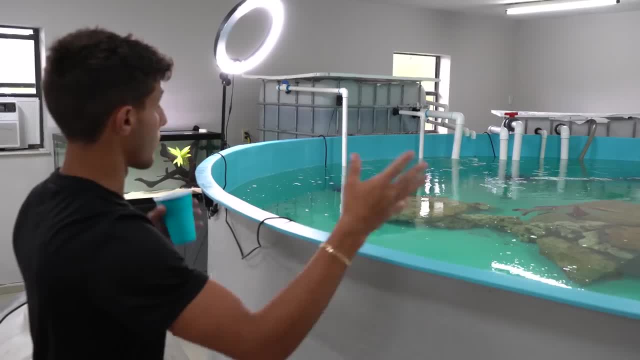 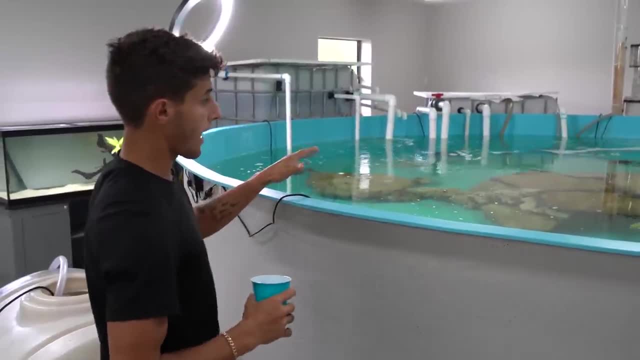 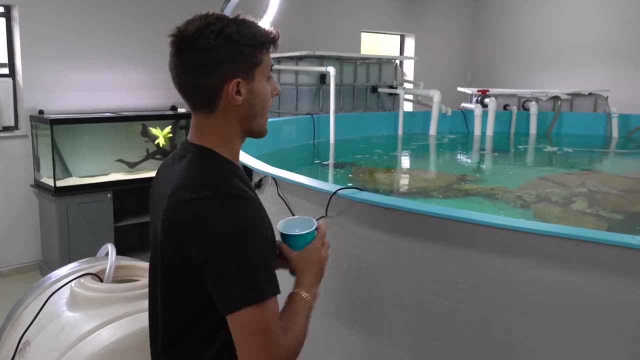 more rock so we can add a bunch more fish. As of right now, I've been just testing things, seeing how the filtration is working without sand and everything's been running smoothly. So as of now, I feel pretty confident adding some more rock, adding sand to the bottom and making this thing. 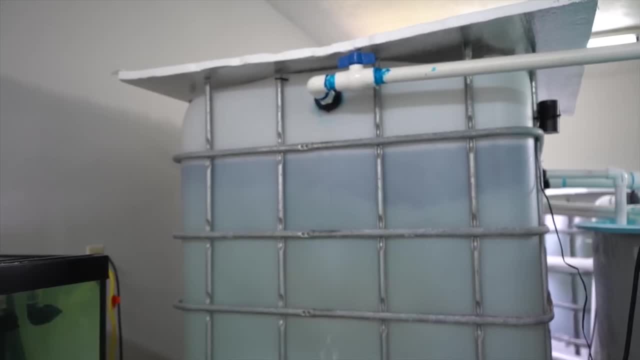 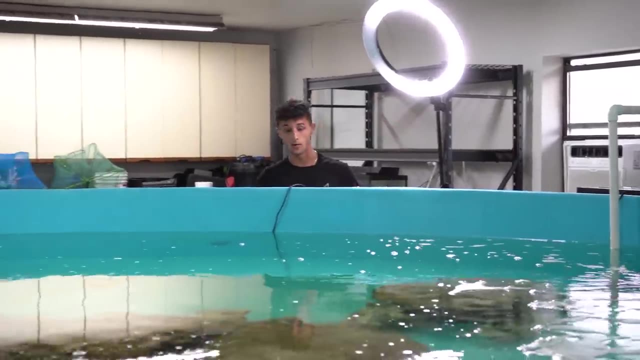 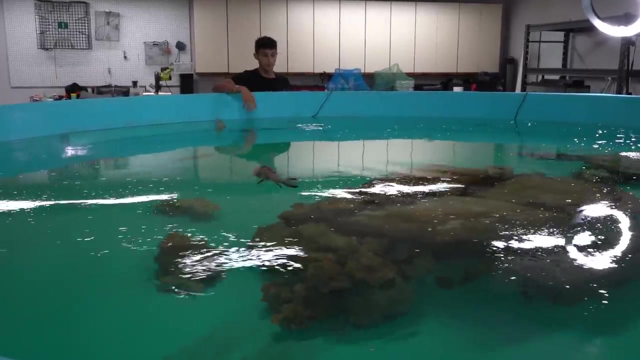 look a lot cooler. We did add another biofilter. We got one right there, another right here, So pretty much double the filtration we had on the last pond. This is double the water capacity, so figured we needed two. We got two filtrations and it's doing its job. This water is crystal clear. Fish are happy, healthy. 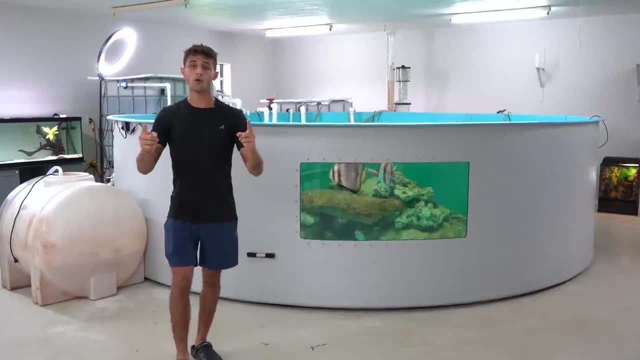 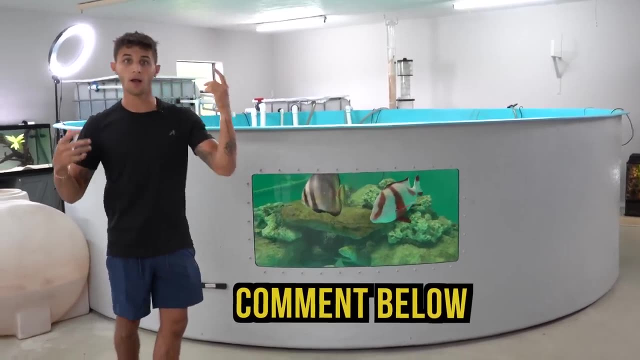 and we'll see what the future holds. If you haven't already, make sure you comment down below what you want to see added to the new saltwater pond. I've asked this a couple of times, but I know a lot of people. new ideas are coming to mind Just seeing it. If you're new to this channel, let me know in. 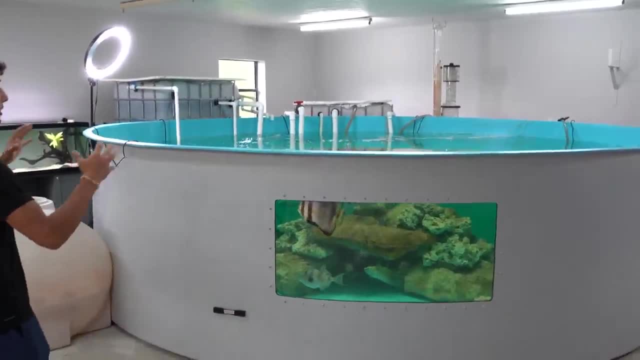 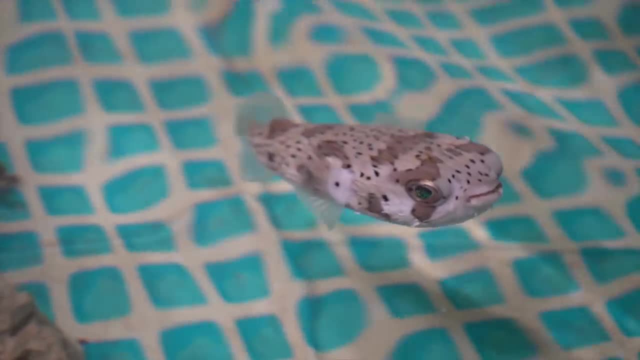 the comments down below, but soon we're going to be adding some crazy stuff into the right. We have our quarantine pond in here. We have our pufferfish crabs. Well, only one pufferfish right now, And I'll tell you why there's. 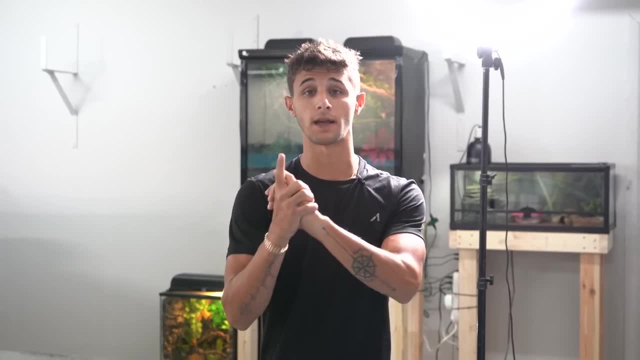 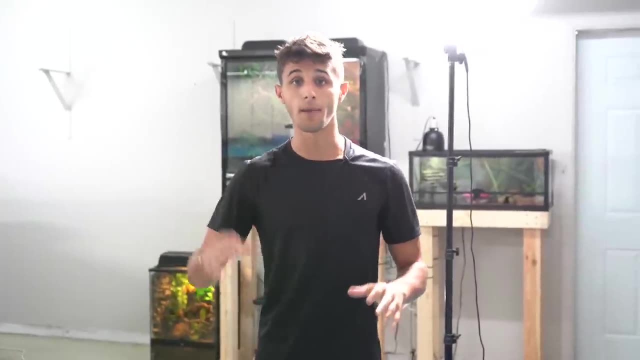 only one. We actually took the baby one and we put them in the aquarium upstairs. We're going to get to that, So make sure you don't skip through the video. but we only added one pufferfish as of right now, just to test everything out. make sure they like the aquariums before we added both And as of. 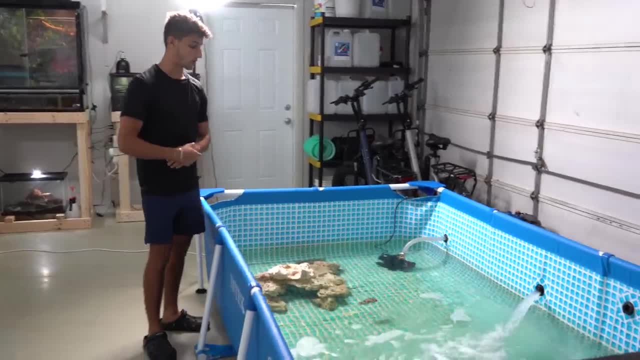 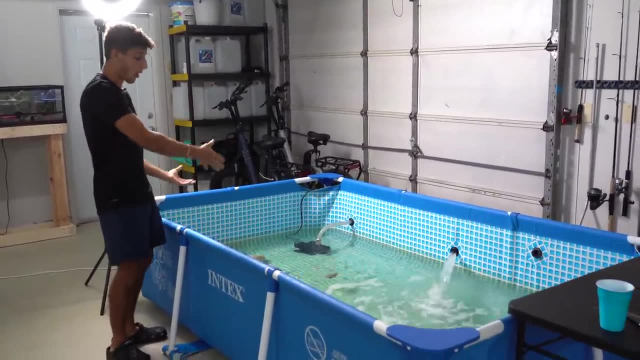 right now he's doing awesome in the aquarium. Sometimes pufferfish don't always do well in aquariums because they see the reflection and they end up like trying to fight themselves and it stresses them out in the pond. They're not able to do that, So we're going to add one pufferfish. 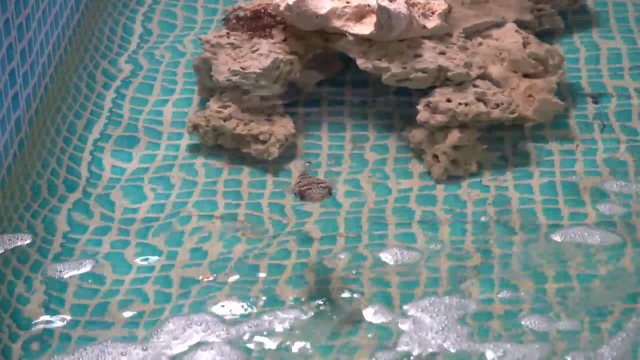 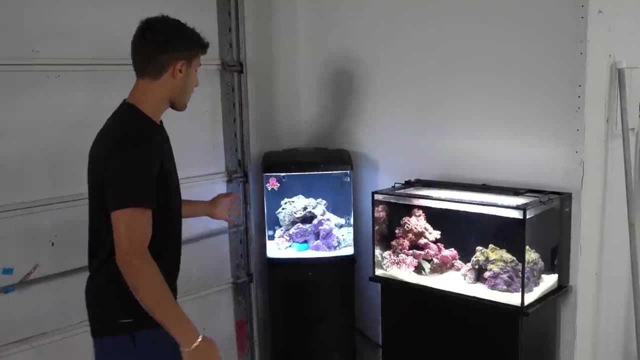 crab, So they're going to be able to do that. So they kind of just free swim, mind their own business and they're not disturbed. Now, right over here, we have our octopus aquarium alongside with our mantis shrimp. As a lot of you may know, I did just post an update on our octopus eggs and 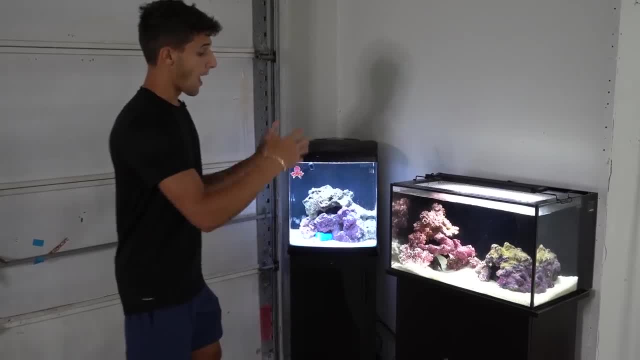 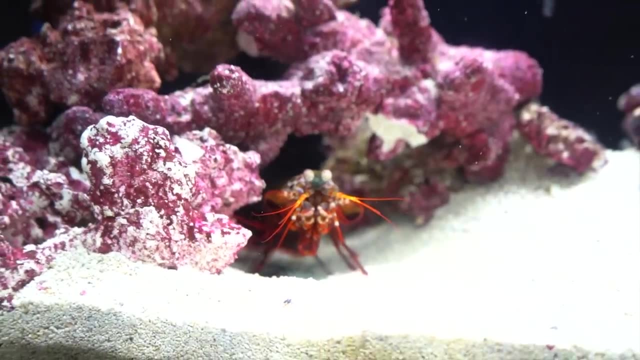 our octopus And I just gave you a rundown of what was going on. As far as our mantis shrimp, this guy is doing phenomenal. He's probably one of the coolest animals we have here on this channel. This little creature right here has the same power as a little handgun bullet. I don't know how well you can. 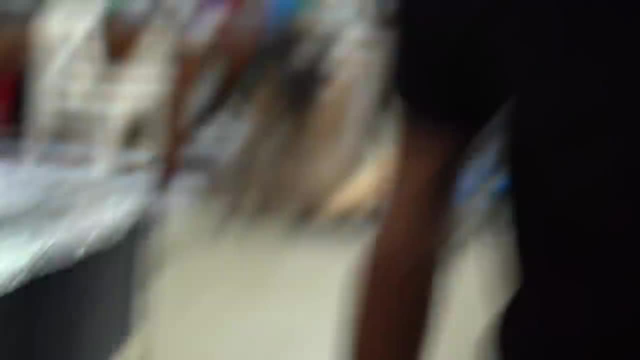 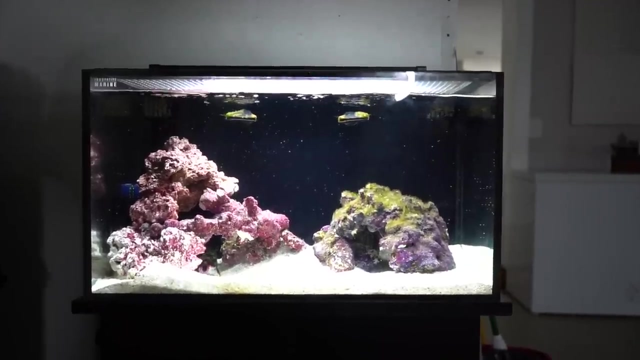 see him right now. but oh, that is exactly what I'm talking about. Yeah, it's just a really cool creature. I did redo his aquarium a little bit. I like to change their states up every now and then, just so they feel like they're kind of in a different environment and they don't get bored. 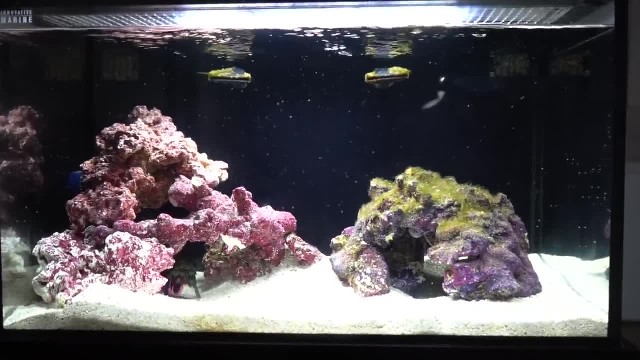 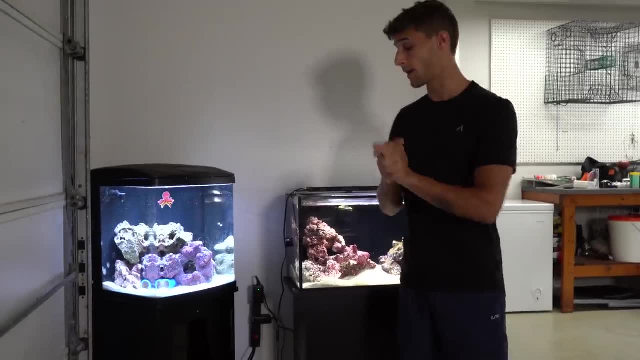 and they end up being very happy. So I do that every like two months. So if you see tanks changed up here and there, that's why. Oh yeah, If you guys want to see a new octopus in our octopus aquarium, let me know in the comments down below. 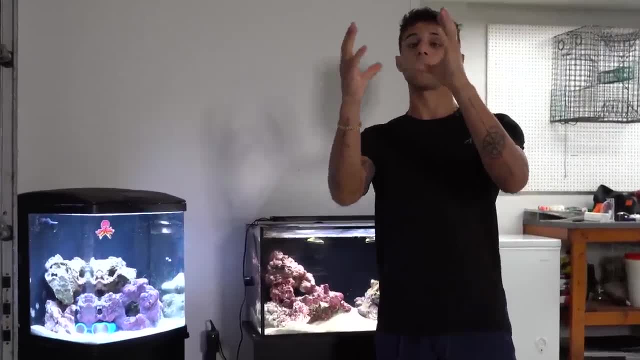 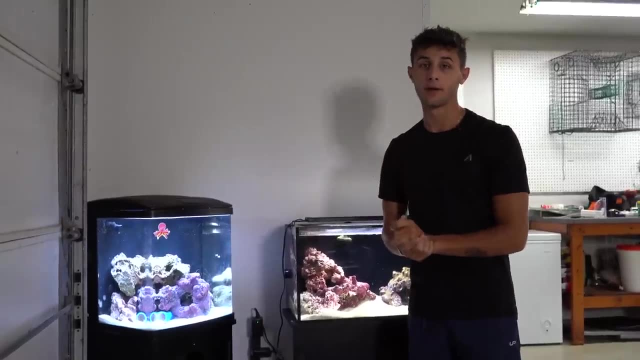 There's a pretty dope octopus out there. I really want to get my hands on one like yay big, We would need a bigger aquarium, but if we can get our hands on something like that, we'll definitely get a bigger aquarium. Now, over to the other side. we did just set up this large rack which is going to 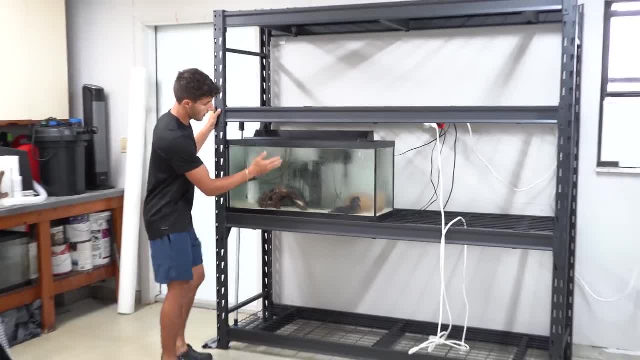 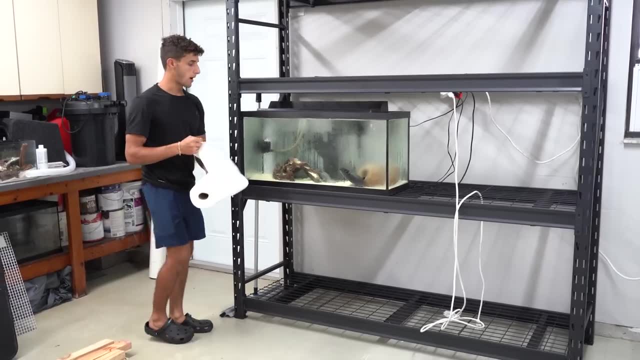 give us a lot more space to add a lot more aquariums. Right here we do have our axolotls. I do have their lights off and I usually keep the lights off. They don't really enjoy it too much, but since we're filming right now, we'll leave them on and show you guys. 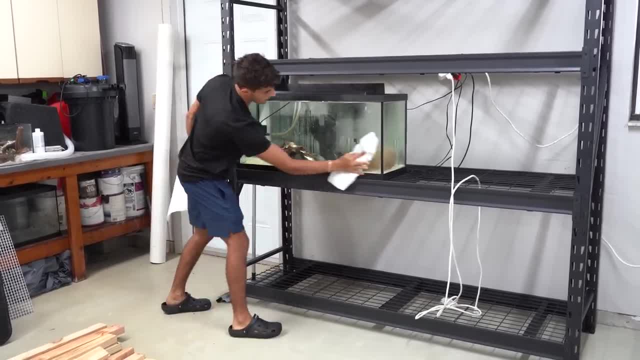 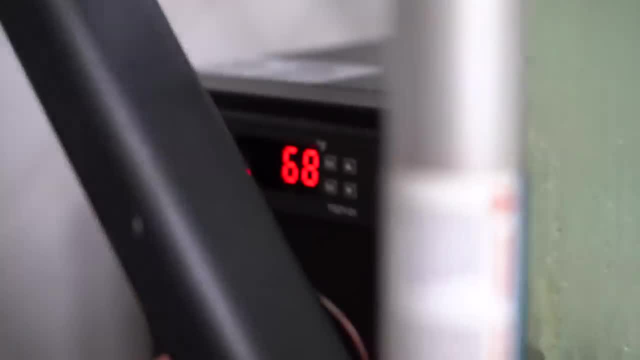 So let's turn them off real quick. You're probably wondering why there's like so much condensation on the outside of the tank. Well, it's probably about 74 degrees in this room Right on the back here we do have a chiller that keeps the water at about 68 degrees, And these guys love cold water. They. 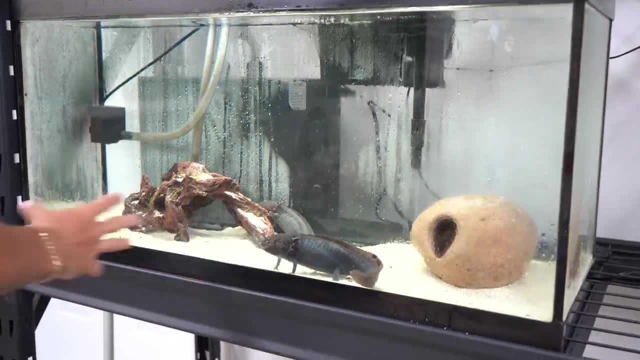 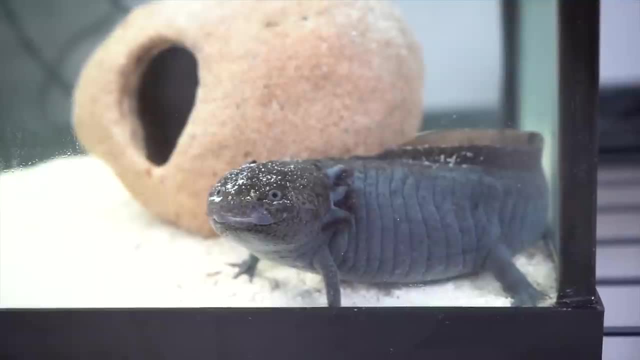 thrive in it. So right here we have our giant axolotls. These guys are probably two of the biggest ones I've seen. This guy we got about six months ago. He's doing awesome. You can see his little chub rolls in there. That right here we got a little bit of a chiller that keeps the water. 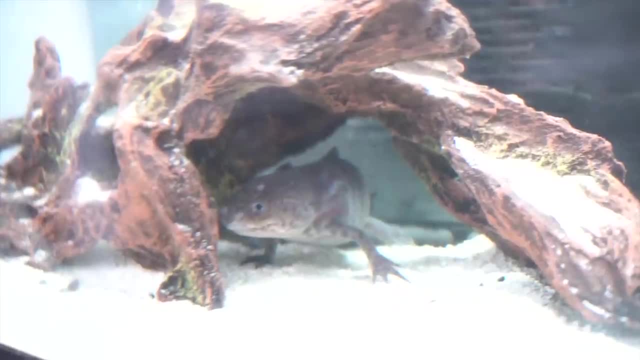 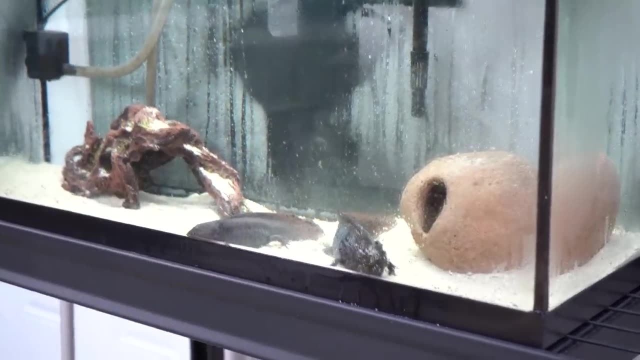 at about 68 degrees. And right there's his little brother who's also doing awesome. He's kind of catching up to him in size, but they're both really, really cool. They eat like monsters and, yeah, they're doing great. I know a lot of you really want updates on our reptiles. It's been. 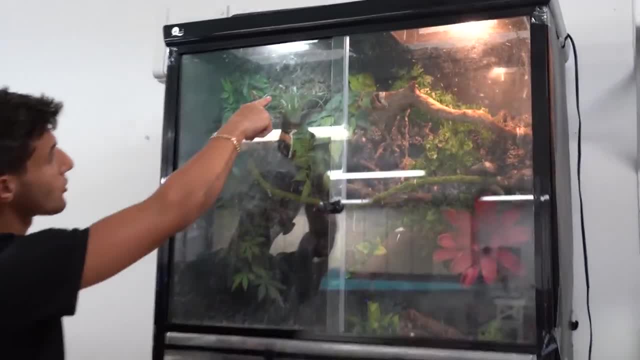 a while since I filmed these guys, but they're all doing awesome. We got our tree python right up there. He is just waking up. It's a little. what time is it? It's 10 o'clock. Yep, He's just. 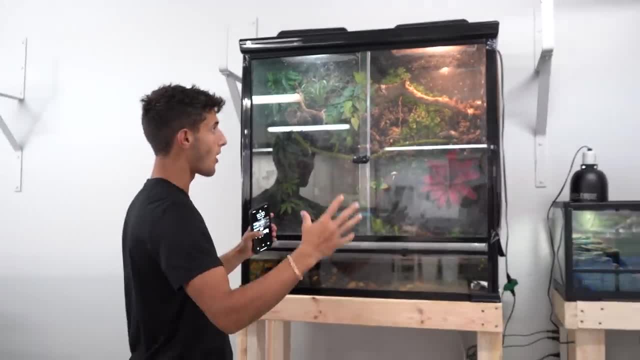 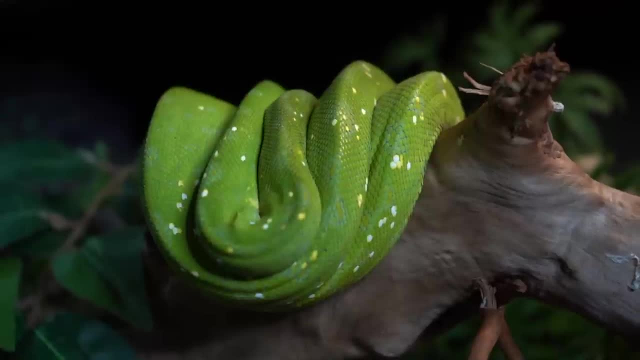 waking up. The lights go on at nine. So once the lights all go on, give him about an hour or two to just come up, realize it's daytime now and you'll see them out and just chilling on the branches. For the most part, though, our green tree python here is nocturnal. I mostly see him active. 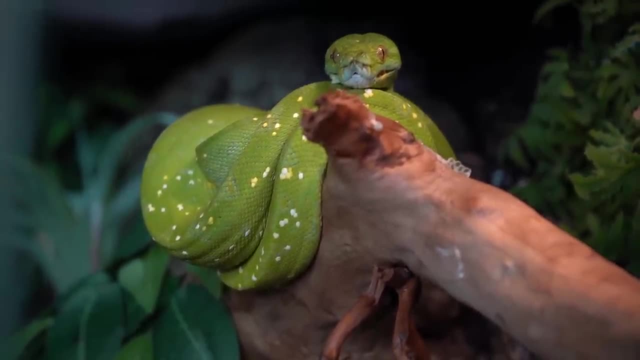 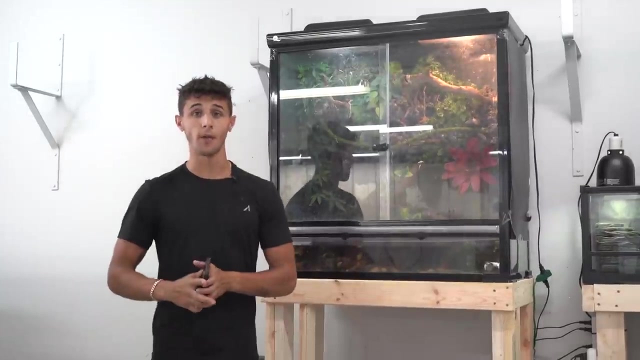 during the nighttime, but there are some times we'll catch him on the logs and stuff just basking, And it's probably one of the prettiest snakes out there. but don't let the beauty fool you. A lot of these green tree pythons are known for having a little bit of an attitude, So 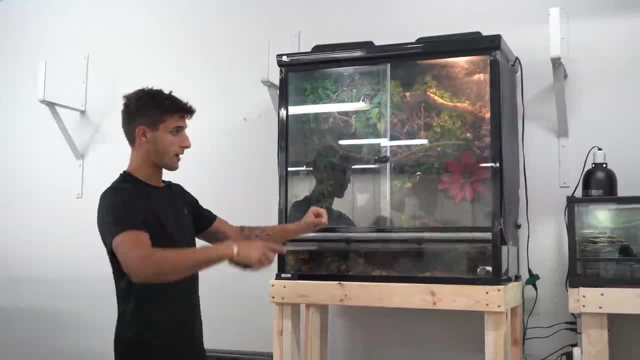 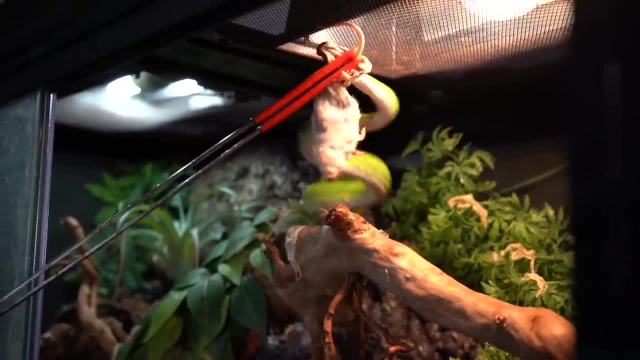 I usually don't pick them up too much. I will with like a snake hook, but when my bare hands they'll definitely bite me. And if you don't know, green tree pythons have some of the largest fangs for a snake. And right below our green tree python we have our exotic Mata. 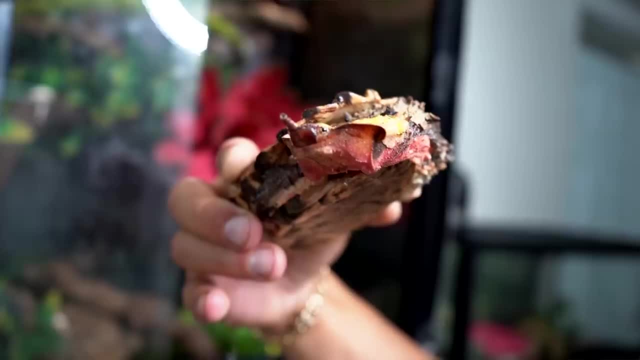 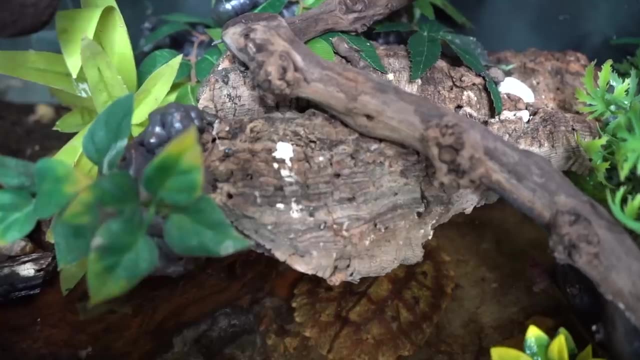 Mata turtle. Not sure how well you can see him back there. He's tucked up in there. These guys absolutely love just hiding up in broken down trees and plants and they kind of just wait for fish to come by and then they ambush it. So that's one reason it's good to have a lot. 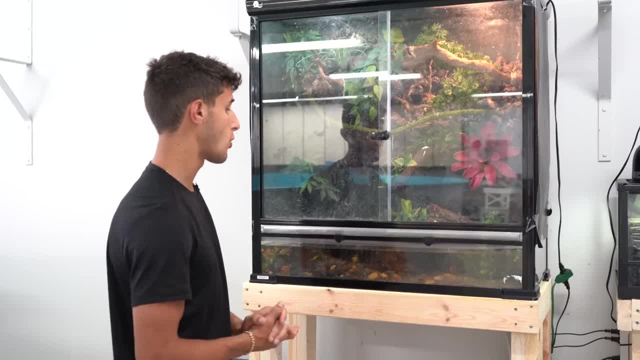 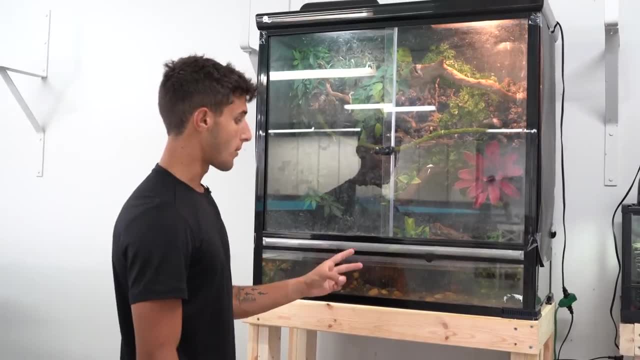 of structure in there. Very soon here, though, we are going to be redoing his aquarium completely and giving him his own aquarium, So pretty much we'll just fill in the whole bottom for the snake and then we'll build the Mata Mata, his separate own like 40 gallon aquarium that he can grow to. 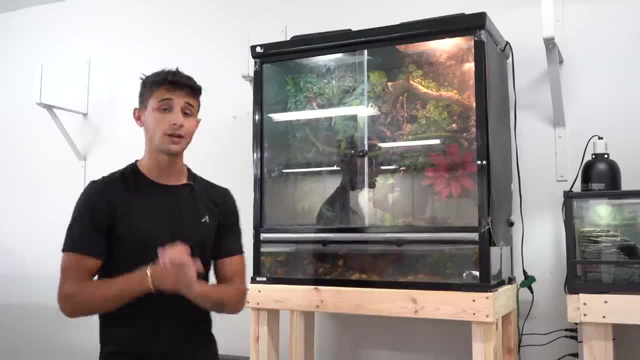 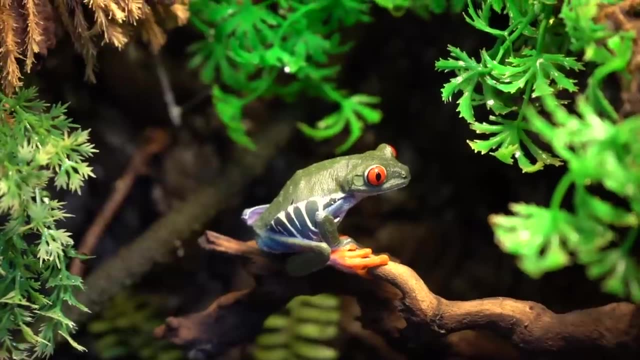 about this big And then eventually we'll build him a nice pond. So make sure you guys are subscribed So you do not miss out on that. Now, right here we do have a red eye tree frogs. I have not yet built a stand for their aquarium, And one reason for that is because I'm thinking 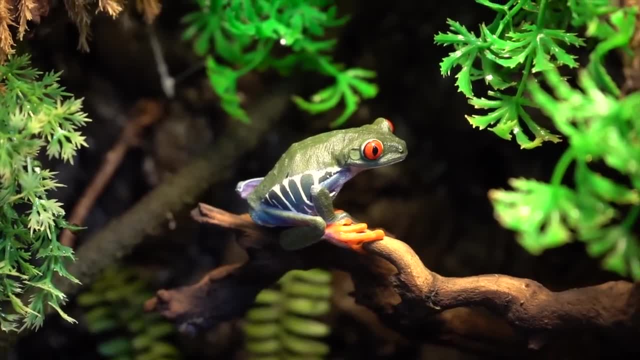 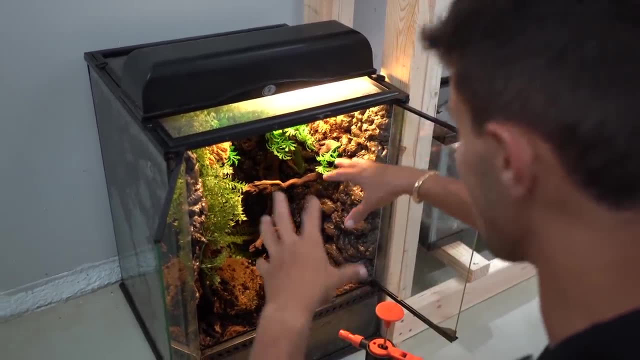 about changing it up, making it more to where we can see them, And that is only because I can never find them when I go to look for them. There's so much places to hide in here. I'm thinking we just make it a glass aquarium with logs and plants, And that way it's kind of like. 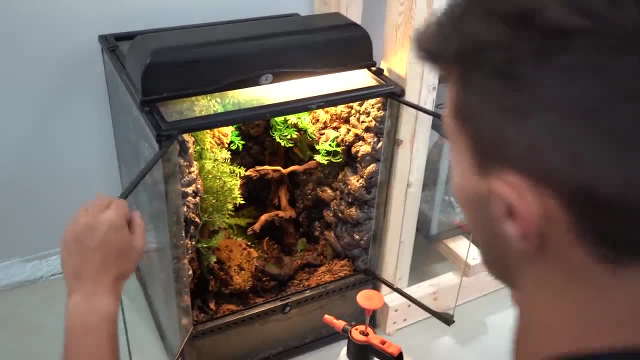 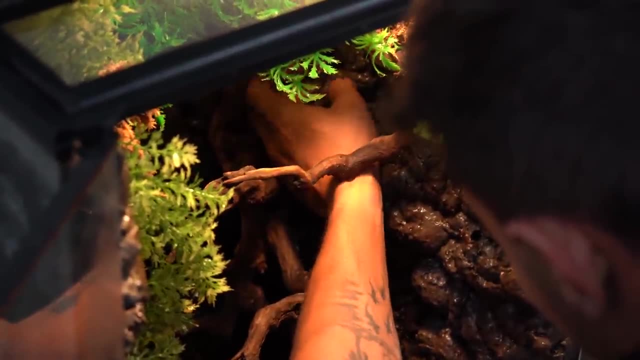 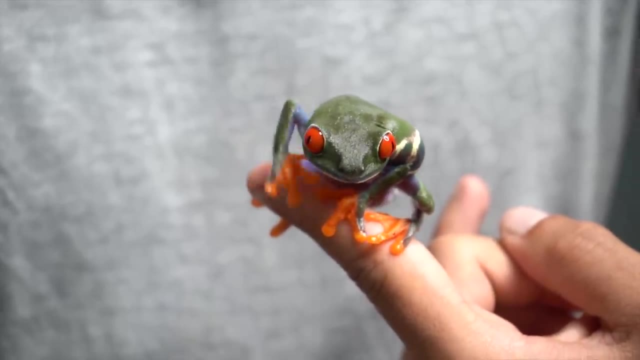 a 360 view. You can always see them, and not just from the front here. but let me wet my hands real quick and we'll grab this guy. right here He's sitting. This is a first, honestly, So you guys are very lucky. Look at how pretty that frog is. It's like it's no joke, man, That's a true. 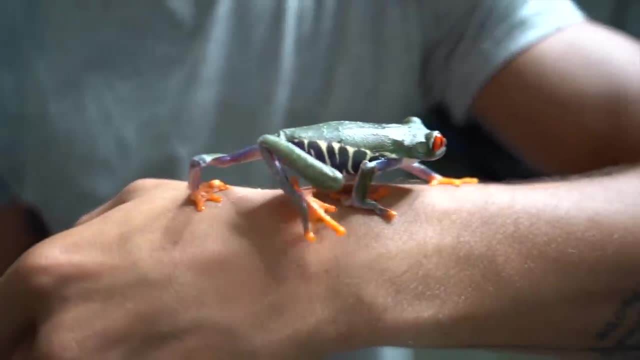 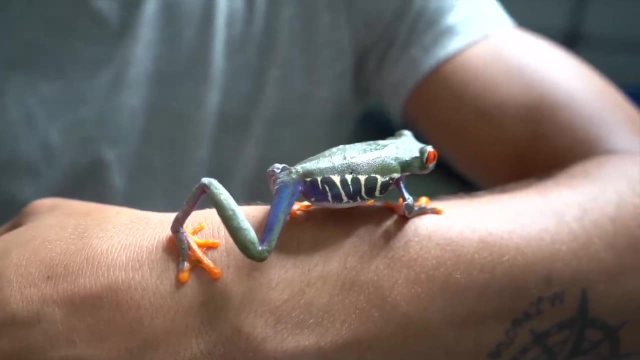 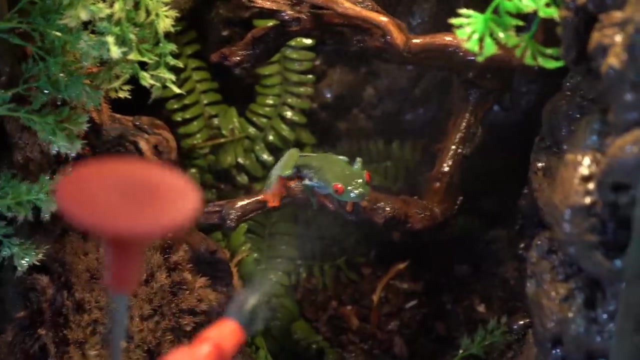 guy Tree frog right there, And we do have two of them. This is actually the larger one. Look at that, bro, Can't lie. That's pretty sick, huh? Just like the colors. like that's God's creature right there, man, So beautiful. He absolutely loves this home But, like I said, we want to be. 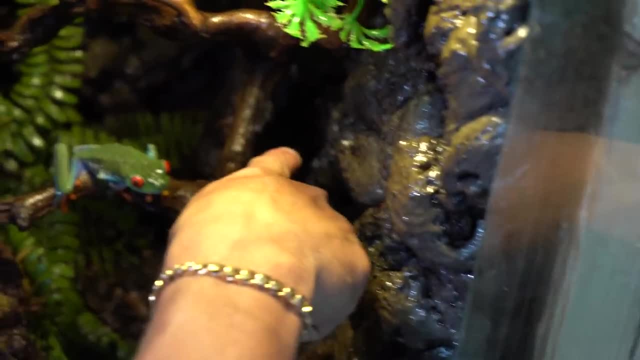 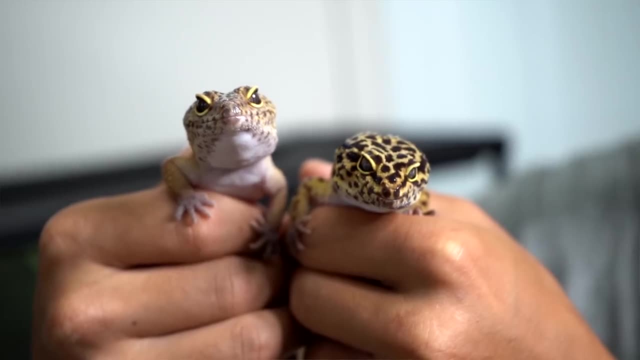 able to see them a lot more. Oh, you can see the little females right back there. Not sure how well you can see, but one's right here and another's right back there. These guys right here are the ones that we got them for about 10 years. Got them when I was like eight years old, which is 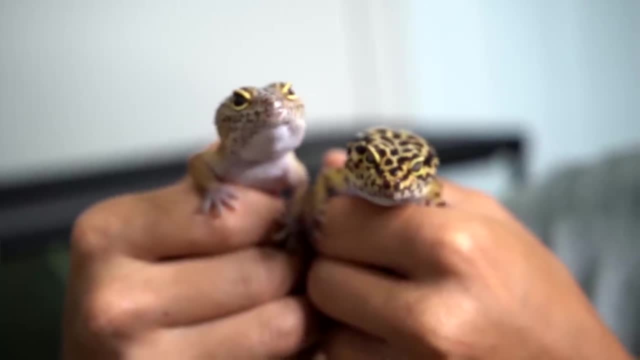 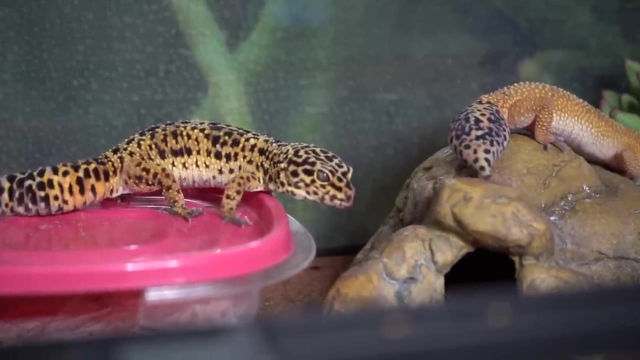 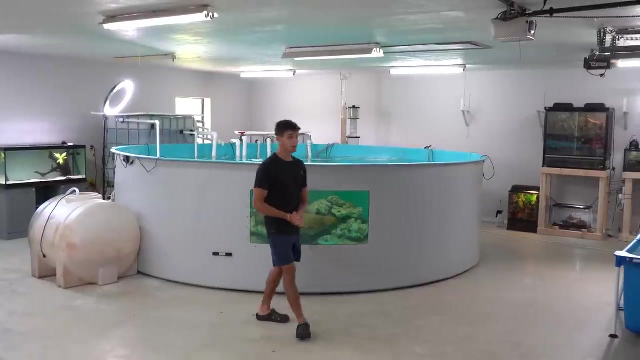 mind blowing. They're still around today. They're honestly one of the chillest lizards out there. They've been living together their whole life, So I don't ever want to separate them. They're literally best friends and they're awesome. Well, that wraps up the fish warehouse. Everything in 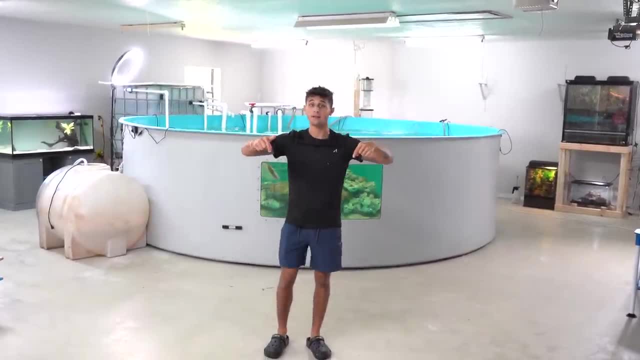 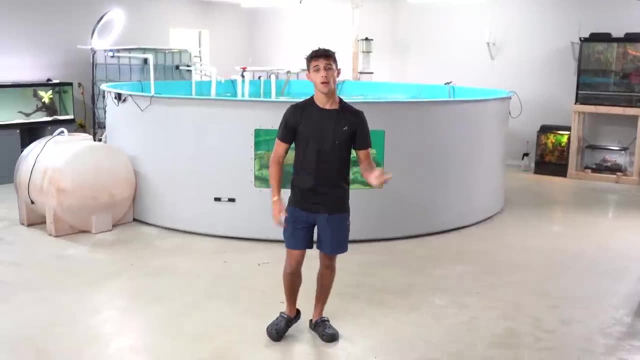 here is doing awesome. If you haven't already comment down below anything new we should get Now that we have our own house with a ton more space, we can do some Awesome stuff. So let me know in the comments down below. but let's keep touring. 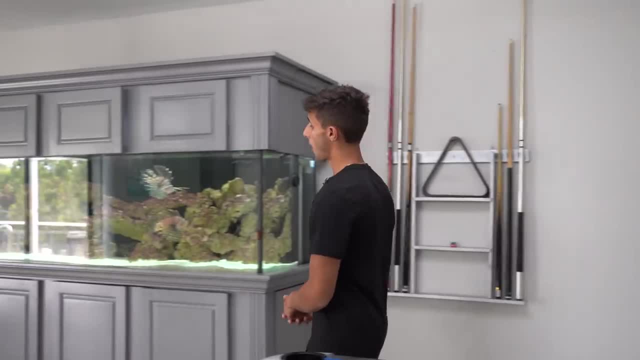 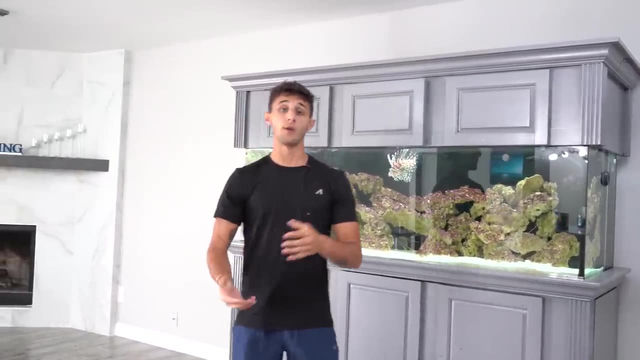 So a lot of you are probably wondering: where is your mini saltwater pond? Well, I'm about to get into that right now. So, as a lot of you may know, we did set up the mini saltwater pond at the last house. We did have to transfer everything to the new house And in that 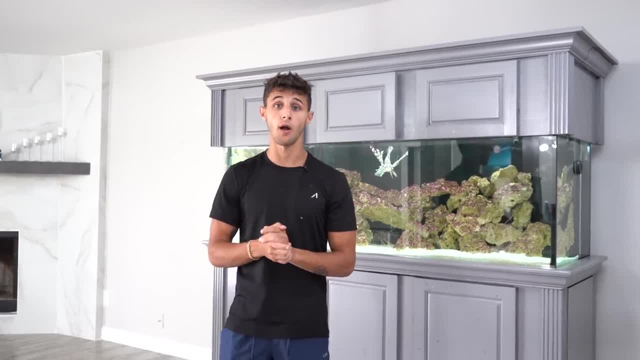 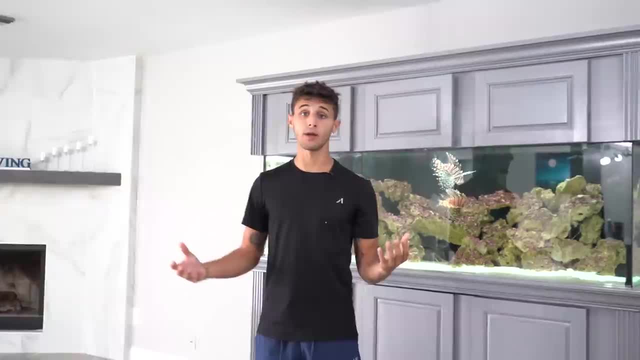 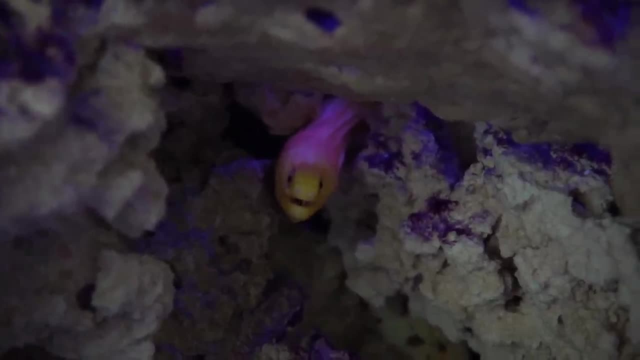 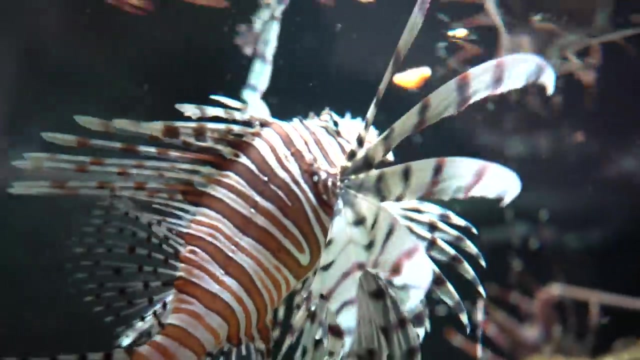 we're going to be setting up a new mini saltwater pond. Now, as far as the 200 gallon, everything in here is doing amazing. We got sunshine, one of the rarest more ales- banana more ales, to be exact. Then we have our two lionfish, along with our two Spanish lobsters, And then, right over here, 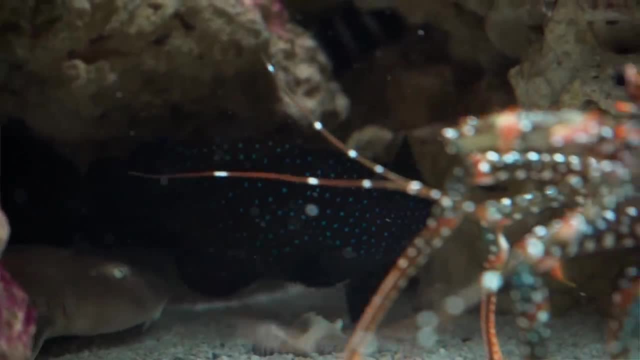 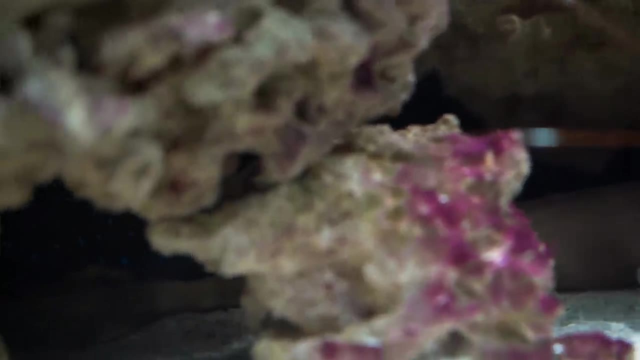 we have our bamboo shark and some are up in those rocks. We have our grouper, And these were the two fish I ended up keeping from the mini saltwater pond: One of our bamboo sharks and our blue spotted grouper, who's somewhere throughout these rocks. 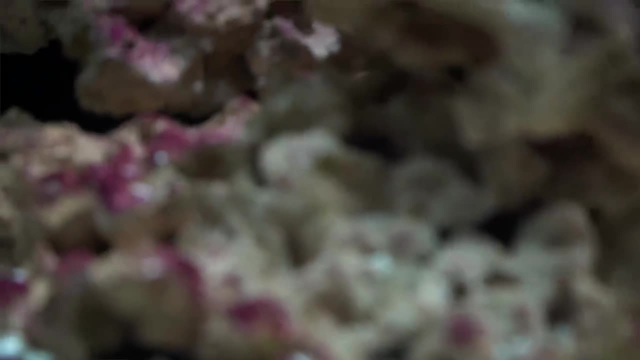 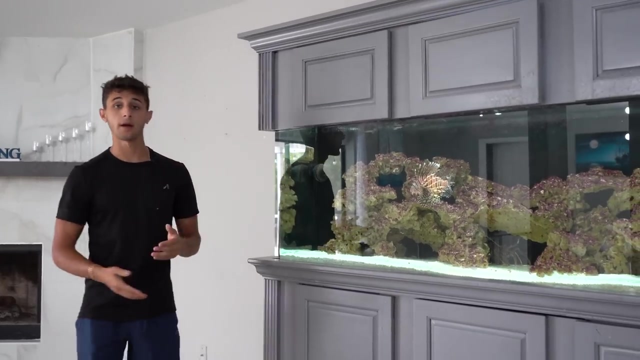 You'll just see them dart out and like eat a fish when food's in there. But soon, once they outgrow this, they'll go into the big saltwater pond. Or if we set up that mini saltwater pond and they're good enough size to go in there, we'll then add them there. But, like I said, we did go through. 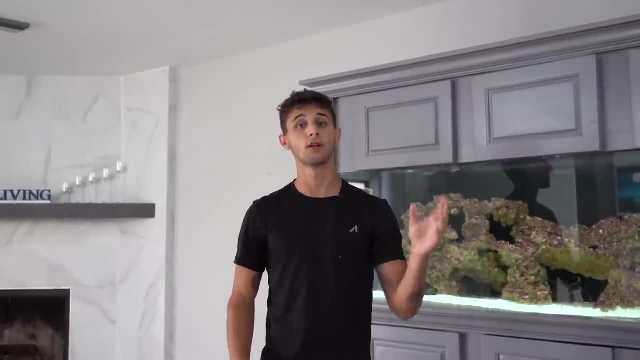 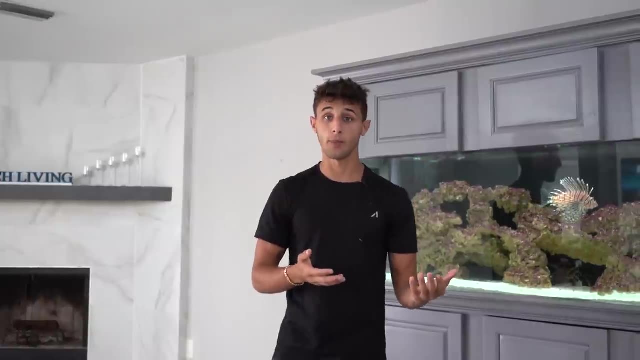 that whole move. It was very hectic. Anytime transferring fish tanks or live animals it's very stressful because not only are you worried about their enclosures and everything, you're also worried about the well-being of the animals. So it's very stressful, but we made it happen and 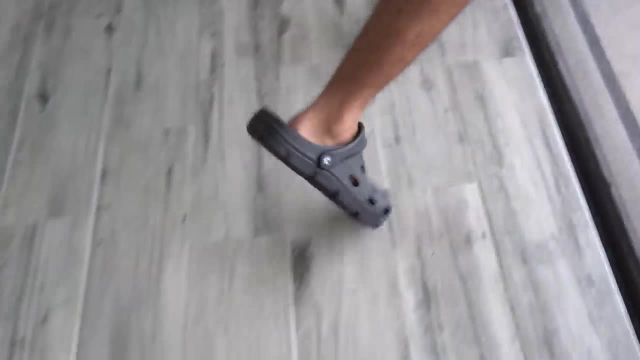 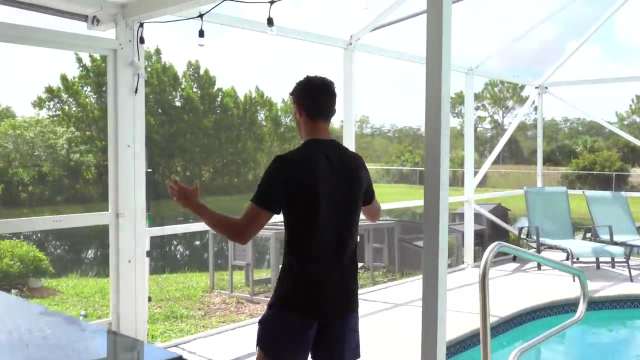 everything's finally getting settled in One of my favorite parts of the house, the backyard. I just love it out here, man. You have so much space. We got so much life back here. Massive pond filled with fish, We got ducks, chickens, and you can actually see there's two ducks right out there. 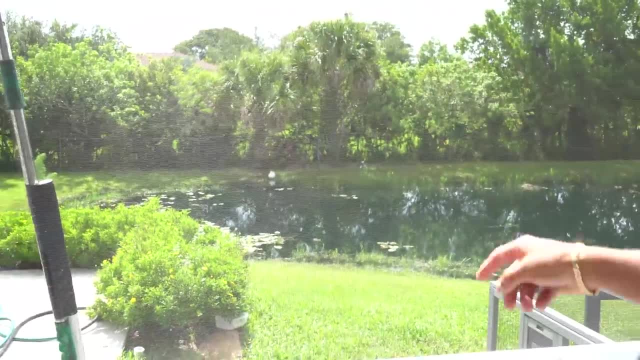 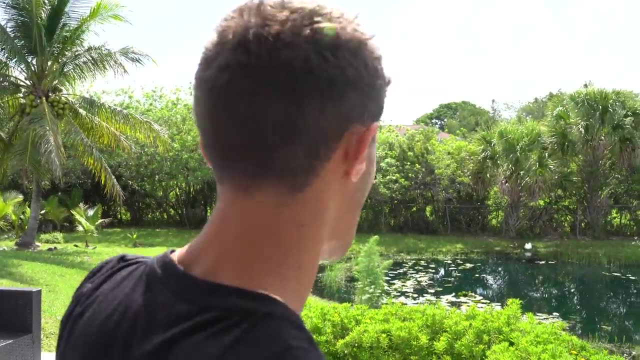 If you guys remember, about three months ago we hatched. There was guys out of an egg. They're now doing awesome. We have two that hang out there. A couple hang out in the bushes over there. It's a little more shadier but this is their home and they're living. 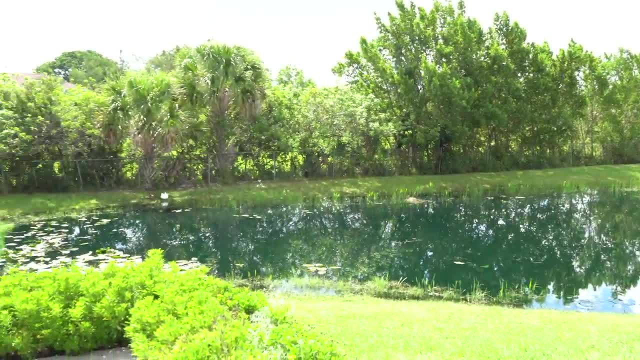 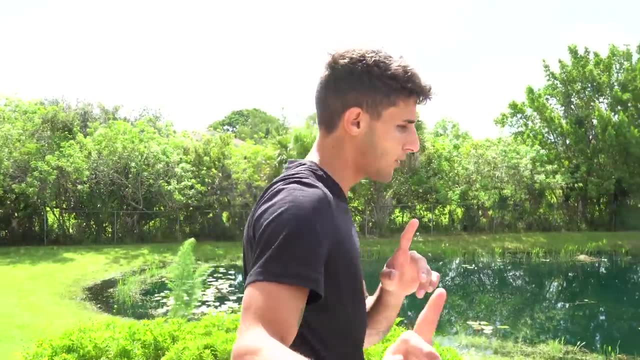 life. Soon, we'll probably add a nice big fountain to this pond just to help with oxygen and movement in the water. But yeah, I got a lot of crazy ideas. honestly, I'll give you a quick rundown of one that I'm really looking forward to, And soon we're going to be doing this. Make sure. 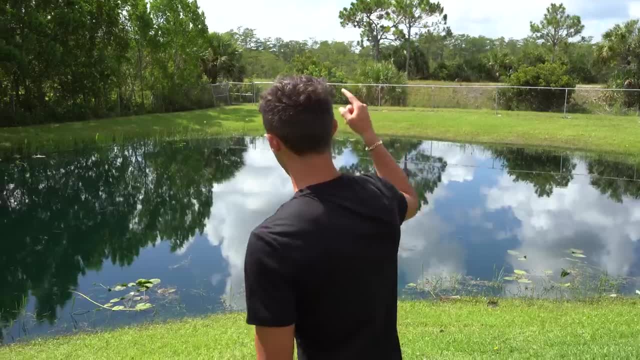 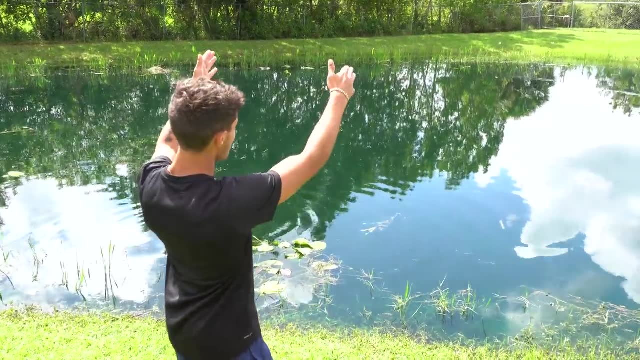 you give this video a thumbs up because I need money to afford this. But right here I want- Oh my, Look at that, Look at right there, We got our koi fish. Right here I want to do a massive dock in the very middle right there and kind of just like a chill. 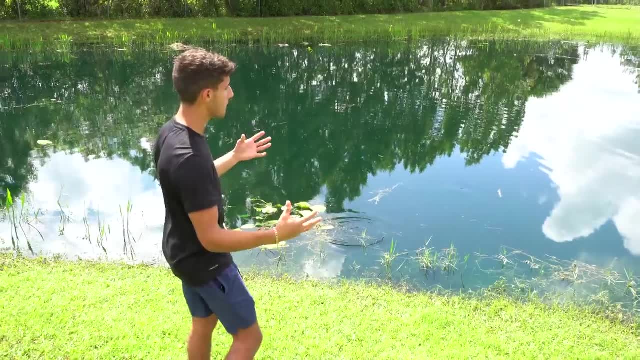 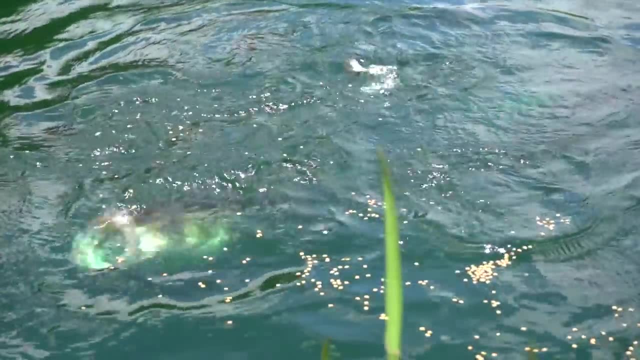 out spot that you can feed the fish. hang out, whatever it may be, And underneath that dock we're going to have a bunch of underwater life. So not only will we be able to film during the day, but at nighttime this place will look insane. You guys are probably like 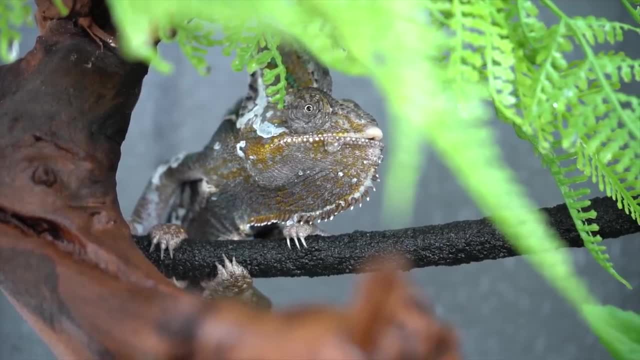 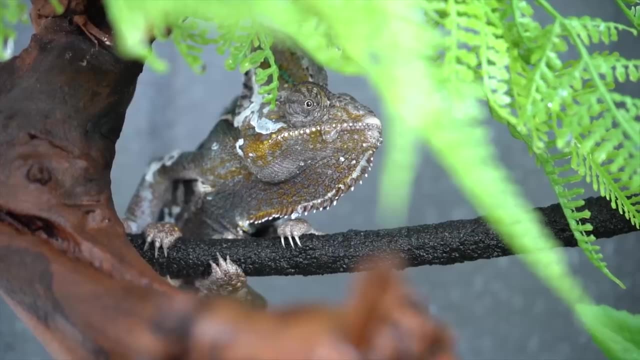 where's Ralph? Well, we actually moved Ralph outside. He's absolutely loving it. It's been about a week since we moved him out here And just having the fresh natural Florida sunlight, along with the humidity and just the warm weather, this guy's thriving You. 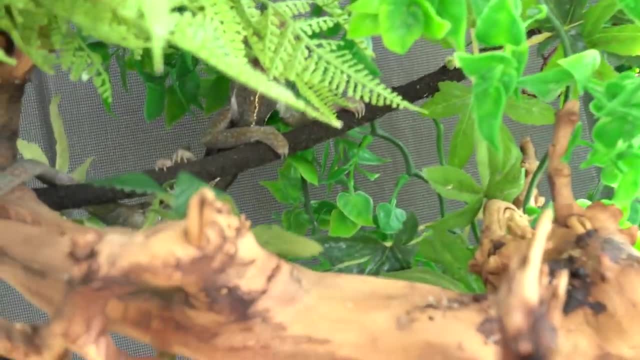 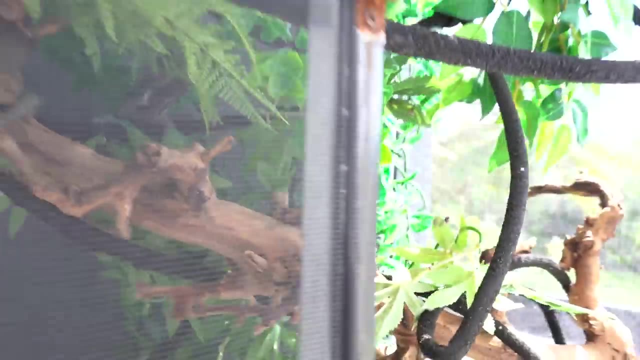 can see him right back up in there. He's a little dark right now. Usually he's really really cool colors But, like I said, he's still adjusting to the outdoor weathers. He is in a screen enclosure so nothing can get to him And he is all safe from predators. 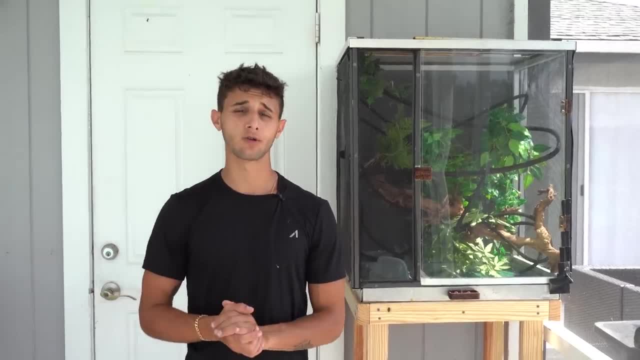 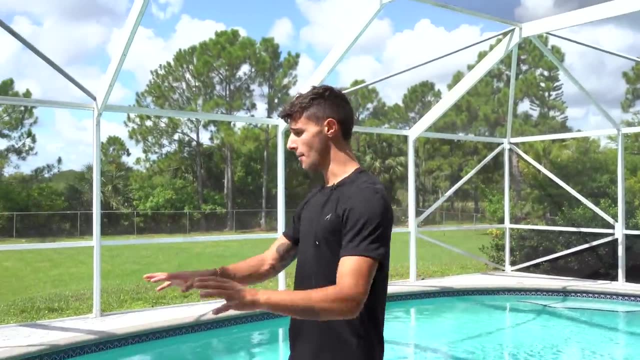 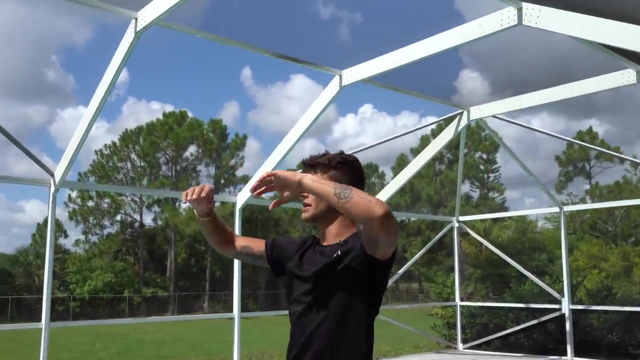 I did mention to you guys that we were going to do an outdoor chameleon enclosure, like a legit one you can walk into. We have this big old screen and we have the pool, So it'd be just like this, minus the pool, and chameleons just free roaming everywhere around you, All vines and cool trees, automatic. 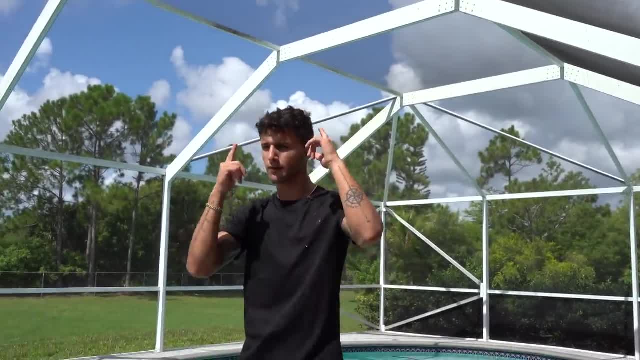 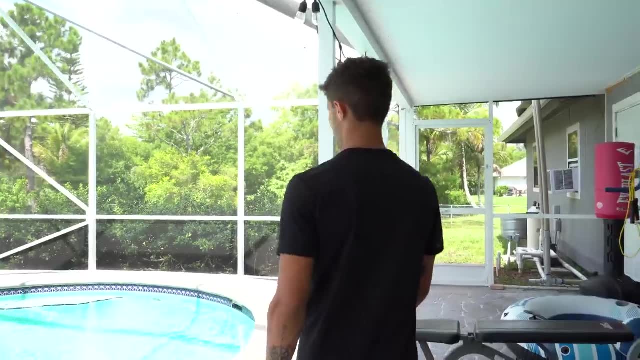 misters from the top. It would be absolutely insane. This is all just a vision I have in my head, but maybe one day we can make it a reality. Make sure you guys are paying attention for this one. This is probably the biggest thing. 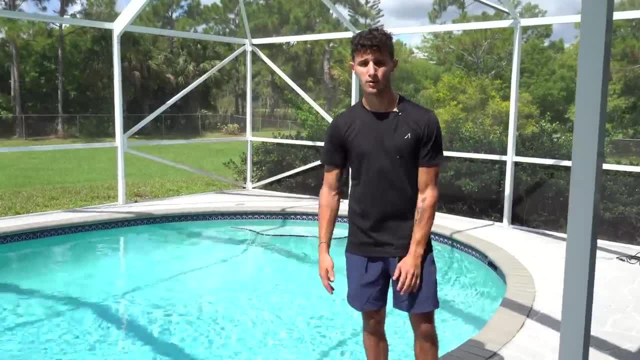 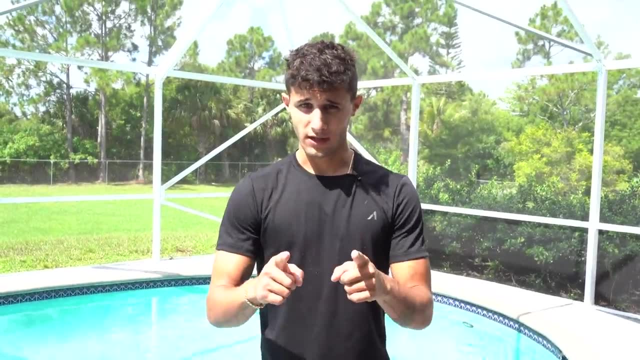 we're going to be doing on this channel- Probably the biggest thing we will ever do on this channel. You ready, I don't know? You guys ready, I don't know? All right, 30,000 likes, 30,000 likes. You're listening right? 30,000 likes, and we are. 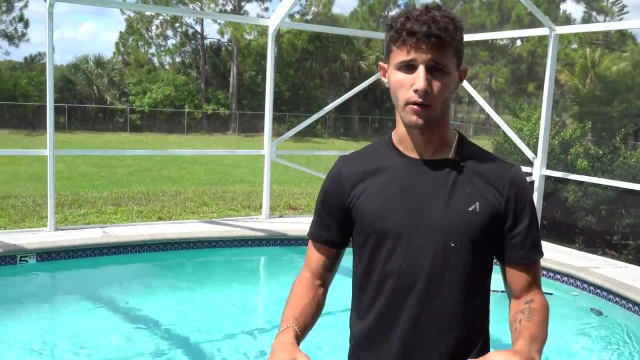 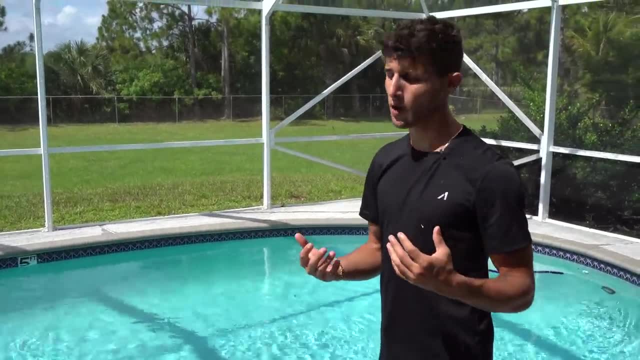 going to turn this pool into a giant saltwater pond Lagoon- Not even a pond. This is going to be a lagoon. at that point, We are going to take all the fresh water out. We're going to have big saltwater trucks come in and fill this with saltwater- And we actually have. 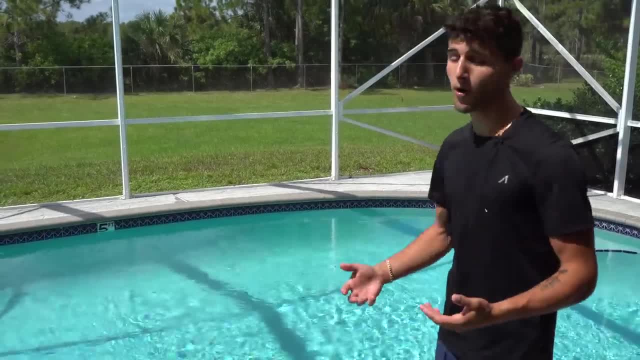 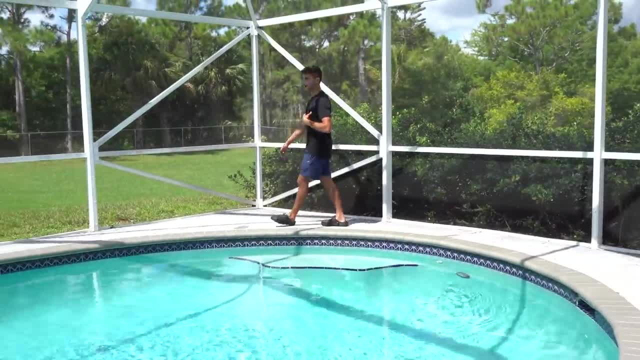 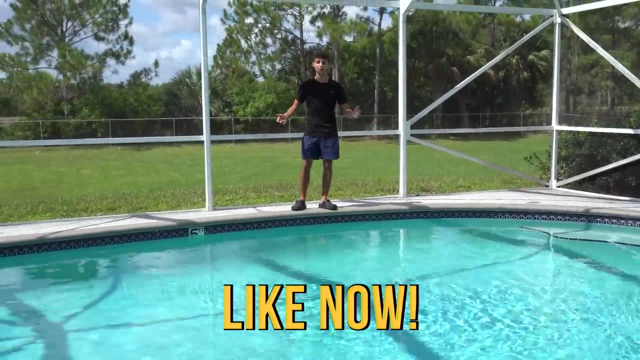 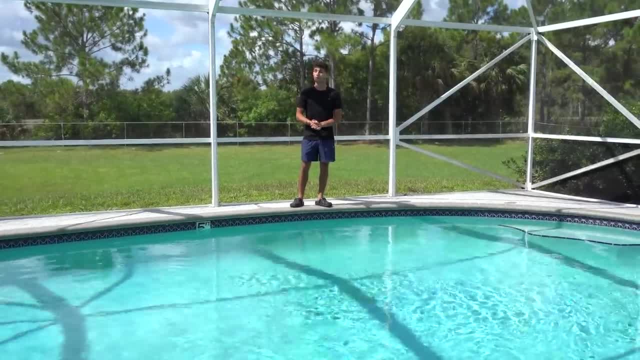 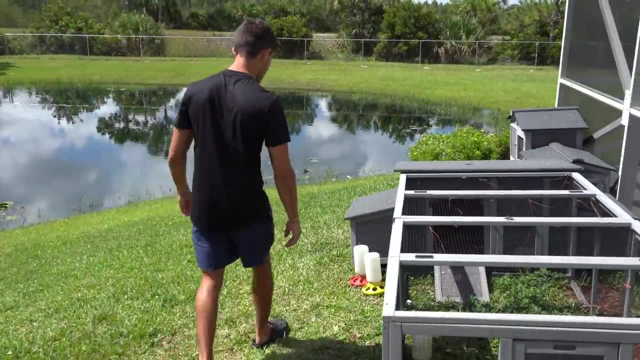 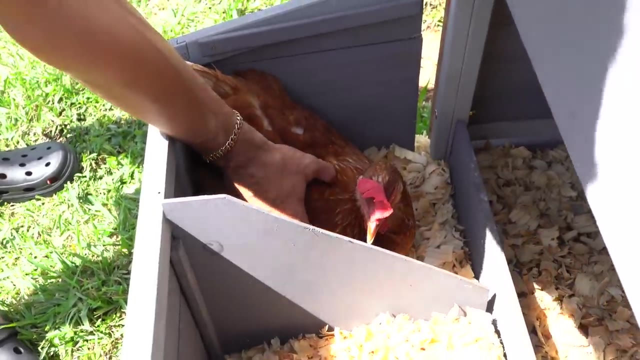 do is hit that like button and probably about two months or a month you'll see this pool turned into a saltwater lagoon. I think salty is on some eggs. here I hear her. Hey, she is, by the way, laying eggs. Come over. Yeah, Look at this, We got two eggs. 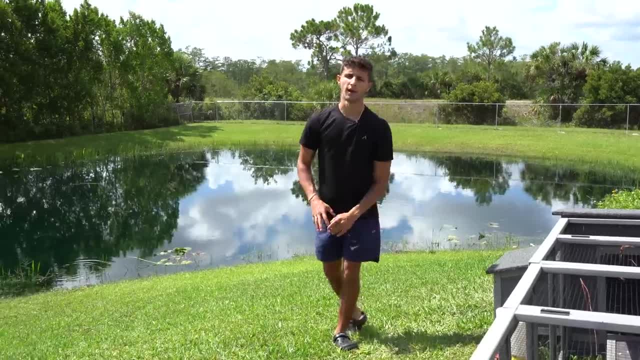 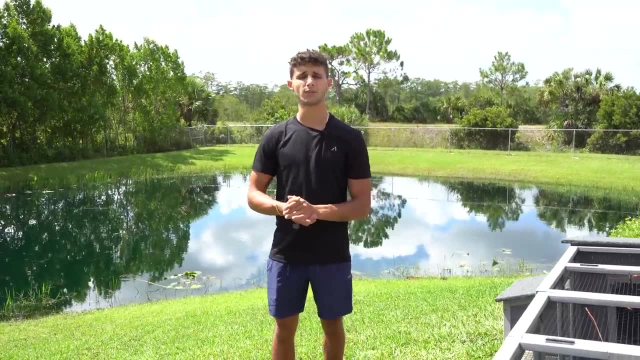 all right, salty's not messing with that too much right now, so we are going to let her be with her eggs. but those eggs are not fertile, so pretty much we just eat them. they're actually really good tasting, a lot better than like the store-bought eggs, um. so yeah, we just come out here. 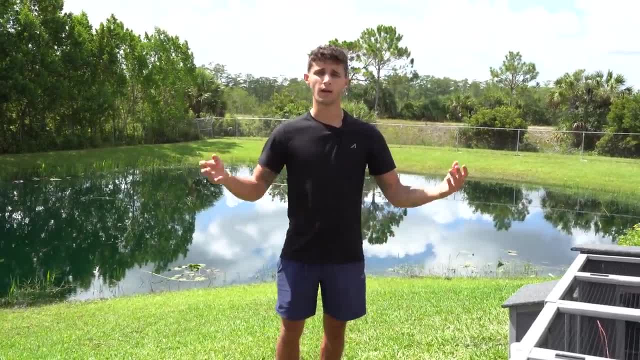 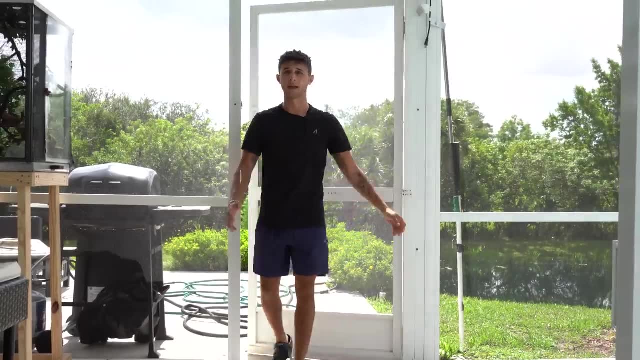 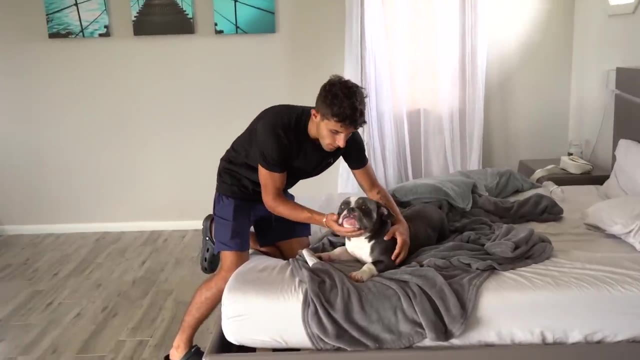 every morning, once she leaves the nest, we then pick the eggs and have a nice breakfast. this property is massive. we have so much space to make endless content, but we do have a couple more things upstairs. let's head up there. room is a little messy, excuse that. but look at this. this. 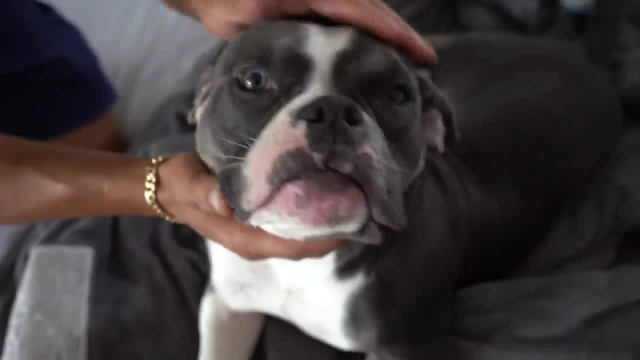 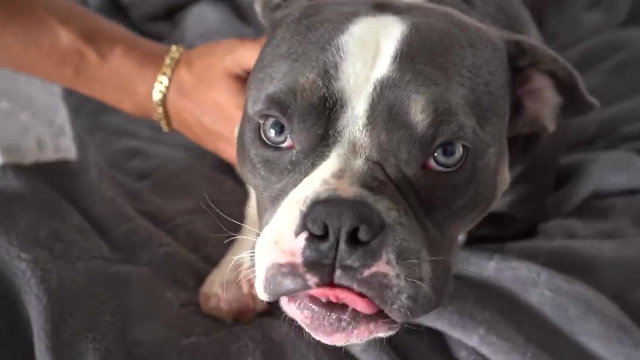 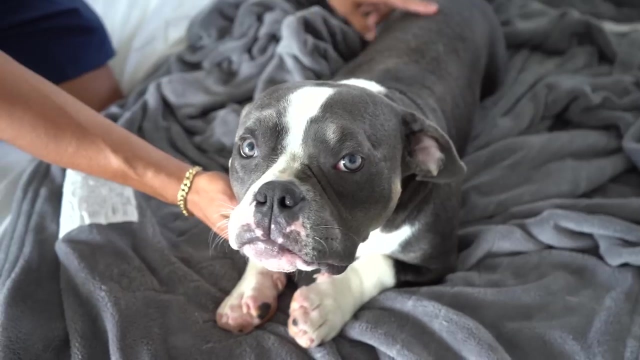 is why it's a little messy right here. this little gremlin meatball just sleeps in my bed. we did adopt this little fella about two months ago. he was, uh, not living the best conditions and ever since he's been with us he's been such a happy little pup doing awesome. fur is actually coming. 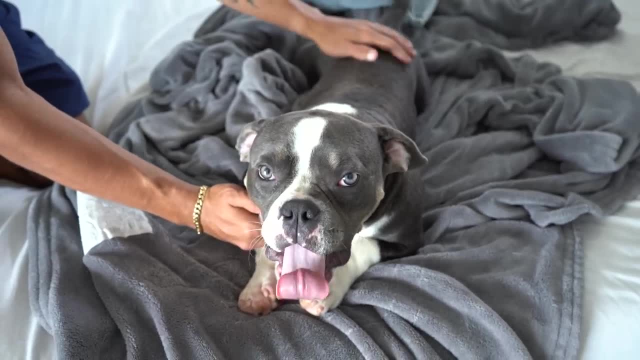 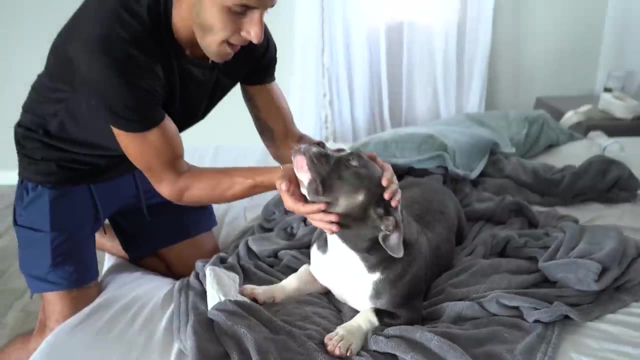 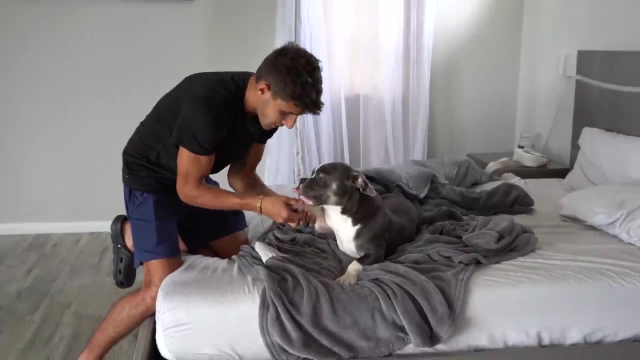 in a lot better. before he pretty much had no hair on his back and that was just from stress and not eating the right food. and now we got him on the right food, we got him living good and he's a happy little bulldog. you're not right, meepo? can you say hi to everyone? what the okay giving me? 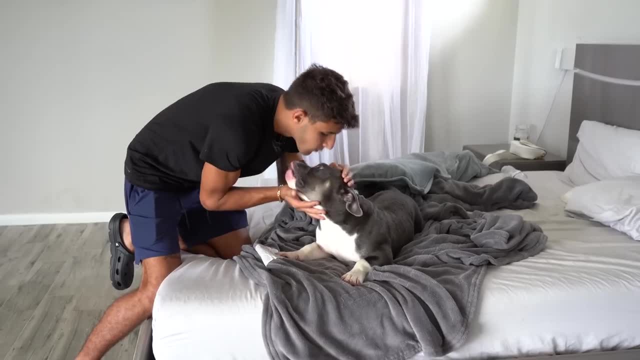 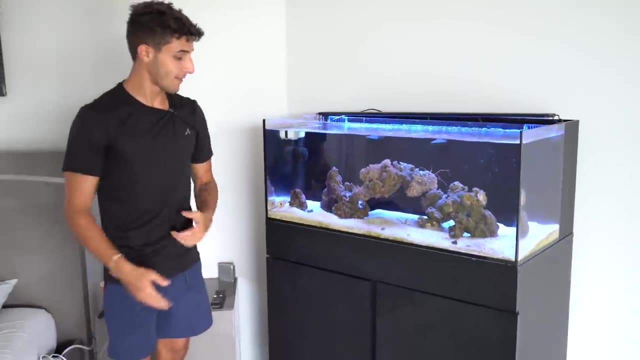 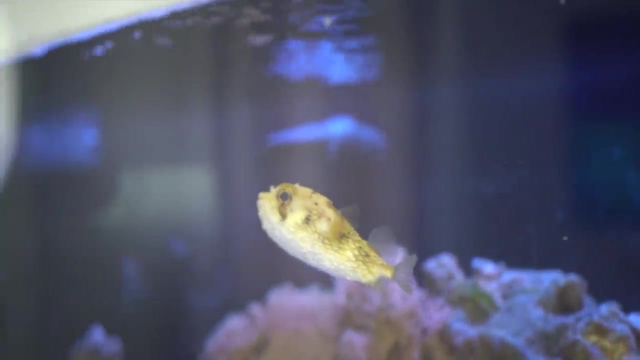 his ma. okay, we love you. we love you right over here. we also have the 40 gallon aquarium and, like i was saying, we do have our mini porcupine puffer- baby porcupine puffer- right here. as of now, he's showing awesome signs. he's been eating no signs of any stress. we do have our panther grouper in here as well. 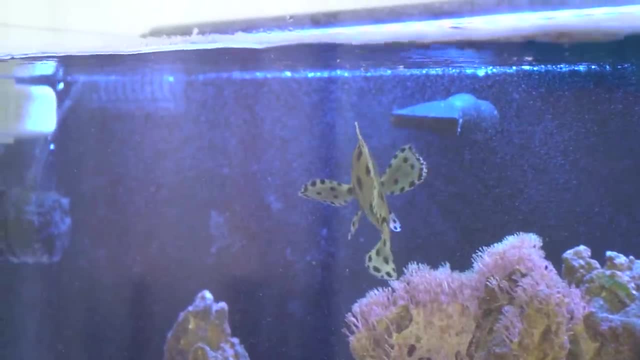 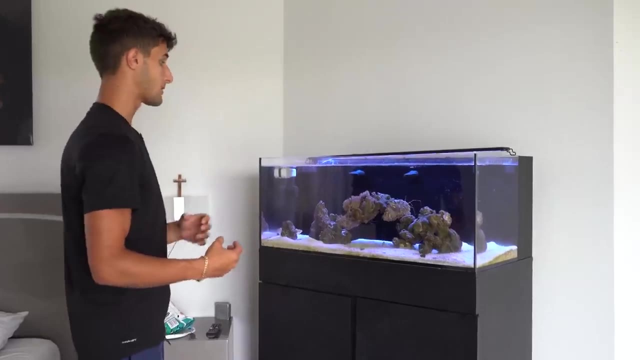 who's also been doing awesome, so i'm probably just gonna have these two guys in here for the meantime. once i see the puffer gets a little bit bigger, he'll then go into the 200 gallon and hopefully by that time we can have our two puffers like reunite and be back together, this panther. 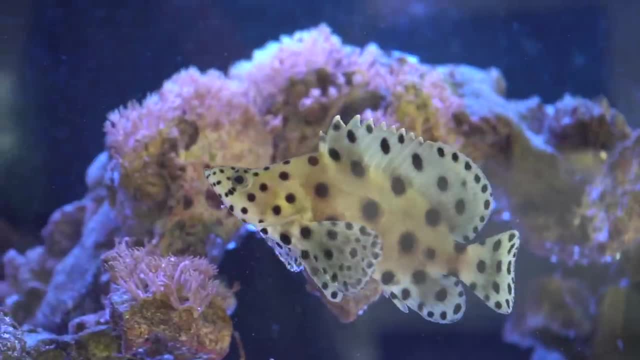 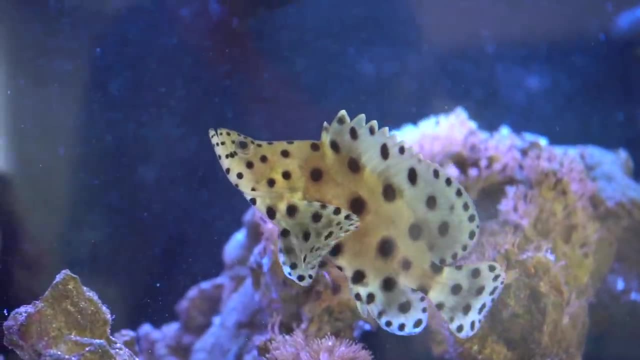 grouper, though i cannot wait till he gets big, because once he gets big he's going into the six thousand gallon saltwater pond and in replace of our old panther grouper. as some of you may know, we did have a disease in that saltwater pond. it is unfortunate, but that's part of the fish hobby. 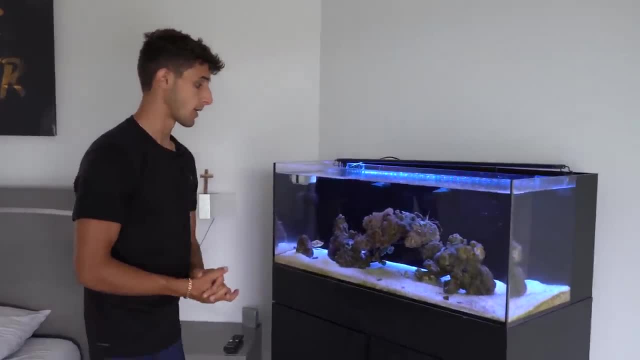 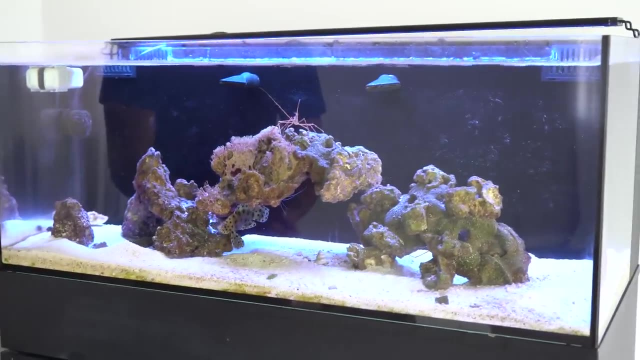 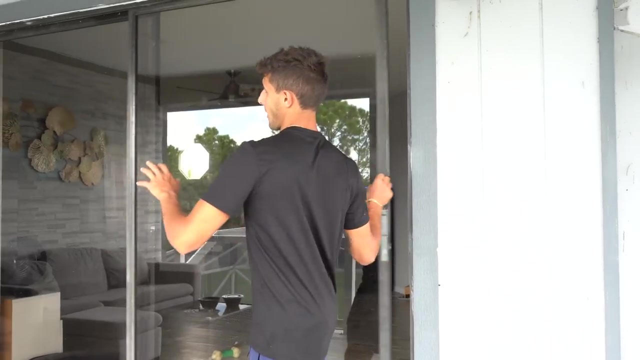 sometimes it's not always sunshine and rainbows. you got to go through some things. obviously it sucks when something like that happens, but that is just part of the game. good news is we now have a baby panther grouper who will one day be massive. this right here has to be the coolest spot in the 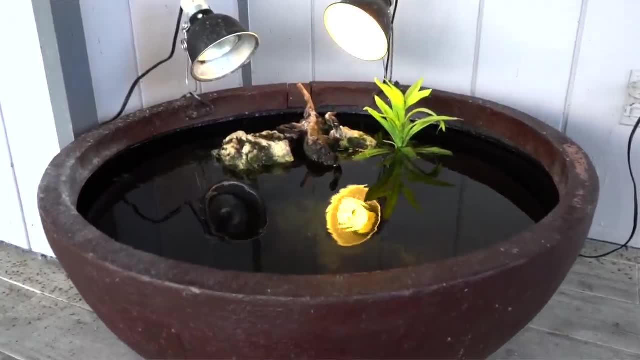 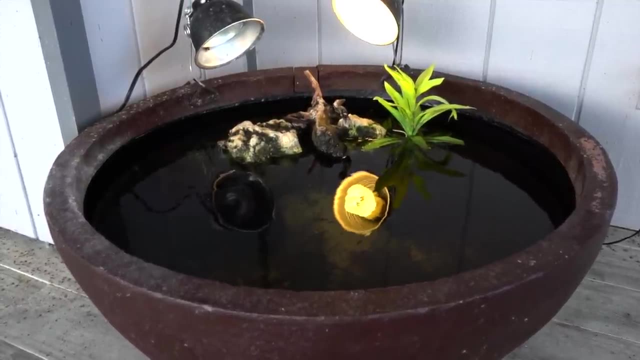 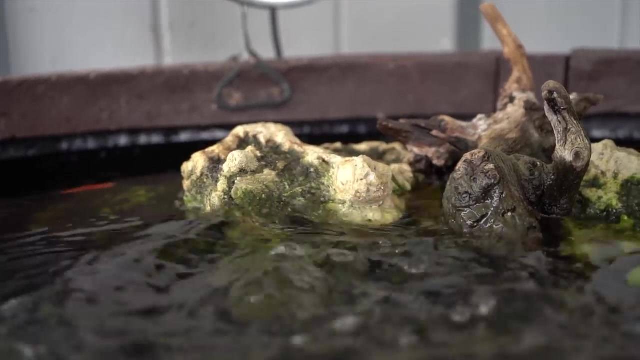 house the balcony. right here is our outdoor patio turtle pond. now i do have some updates to give you about these guys, but as of right now, all we have in here are our two pink belly side neck turtles, our african side neck and our two yellow bellies we did end up releasing into the backyard pond. i 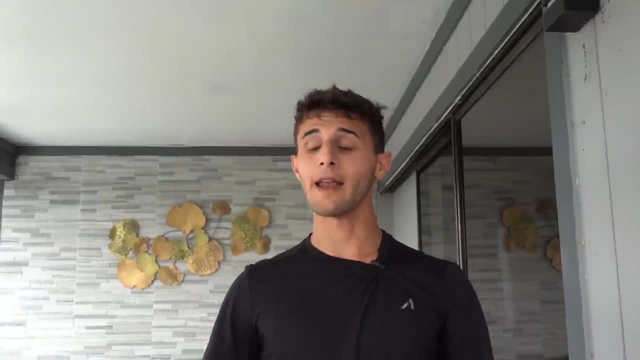 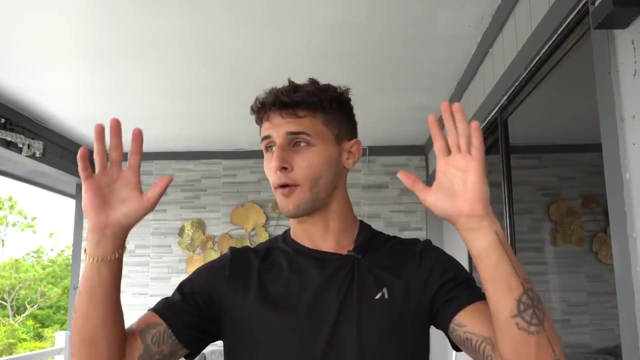 am really bummed out that i didn't film it. sometimes i just get really excited and i end up just doing it and not realizing i got people that want updates, so i apologize about that. anything from here on out i will film. like anytime i put something into that pond, i'll make sure i just 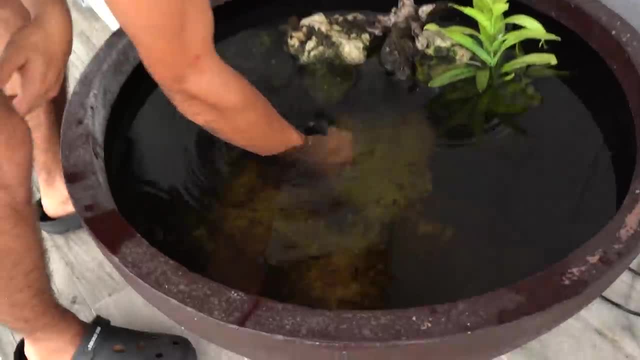 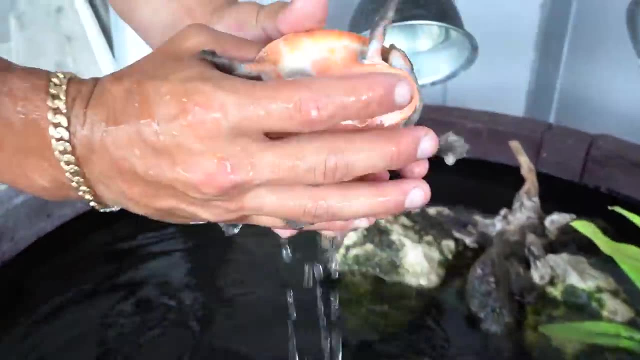 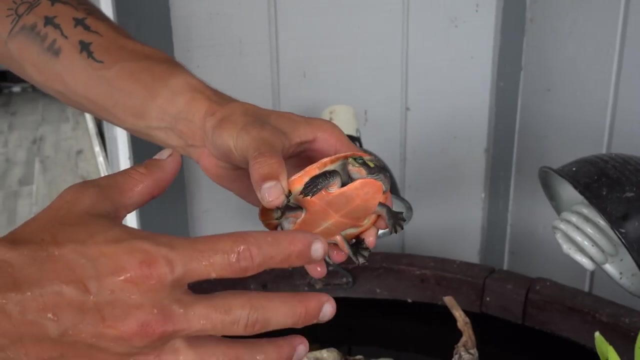 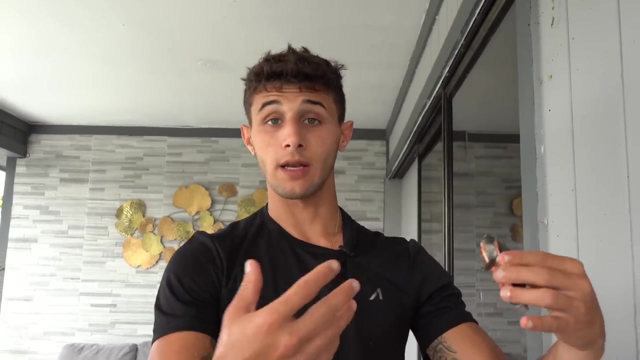 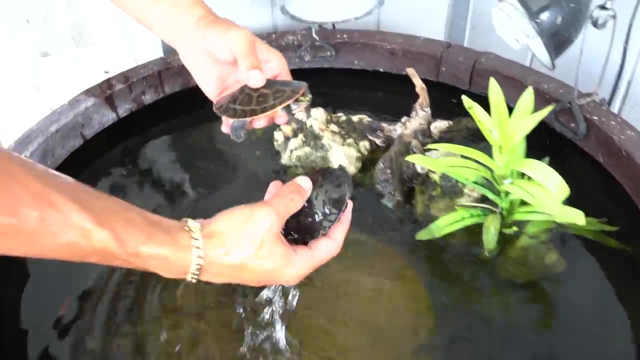 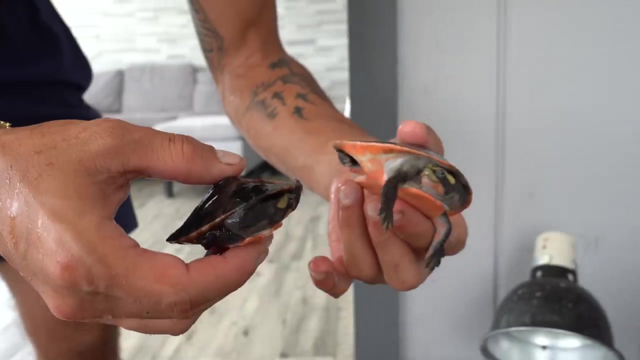 you know, film it real quick and then add it to a video later on. but let me know what you guys think about it and i'll see you guys in the next video. a lot bigger than this guy, but we got them at the same time. some of them just grow at different. 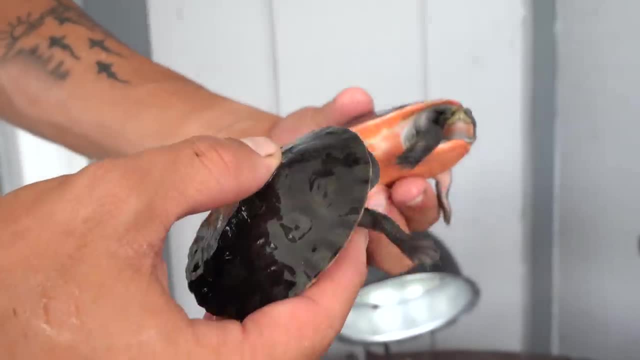 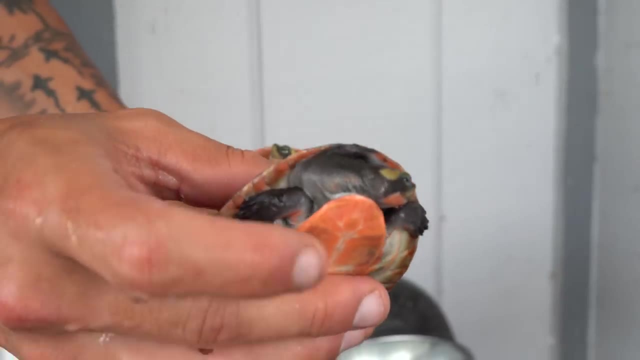 rates. this guy may get a little more food than this guy, but um, awesome turtles. you can see why they call them side necks. instead of like a regular turtle bringing its head in its shell, it just puts it to the side there. so that's how they get their name.